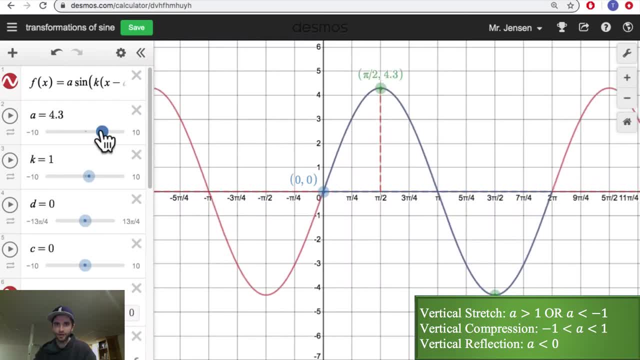 Desmo. So as I manipulate a, notice that the sine function I have here is being vertically stretched or compressed, and notice if I make it negative, it also does a vertical reflection Right. so if a was four, it's a vertical stretch by a factor of four. If a is negative four, it's still a vertical. 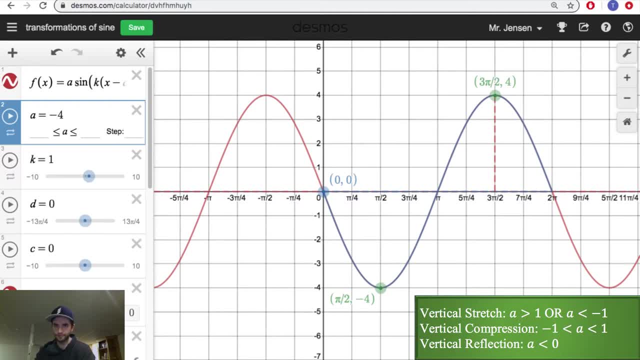 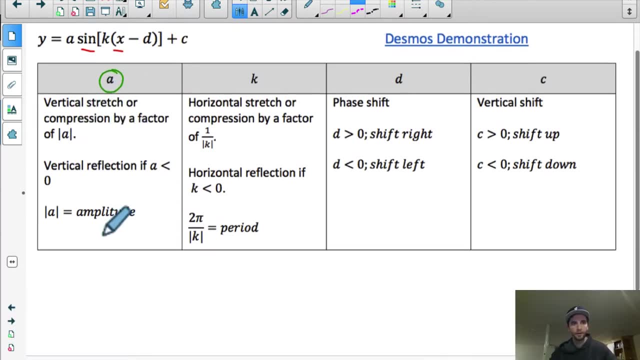 stretch by a factor of four, but it's also been vertically reflected, So that's summarized in the table right here. Vertical stretch or compression by a factor of the absolute value of a. It would be useful to note here that it's a vertical stretch if a is greater than one or a is less. 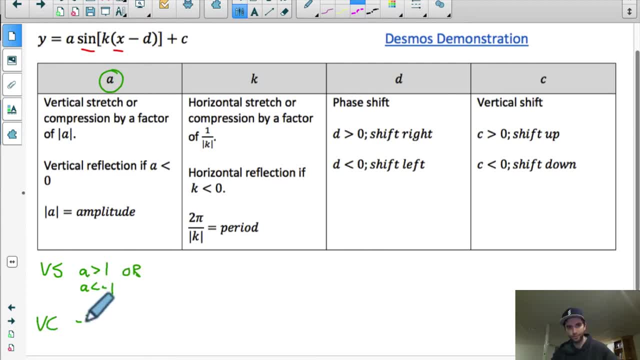 than negative one, and it's a vertical compression. if a is between negative one and one, And it's a vertical reflection if a is less than zero. meaning if the a is less than zero, it's a vertical reflection. If a value is negative, there's also a vertical reflection. Another thing we should talk. 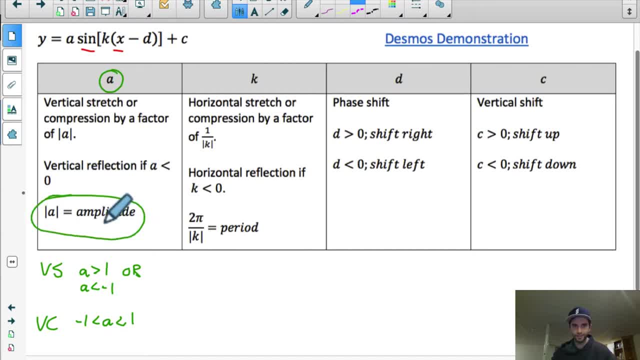 about is that the absolute value of a actually very specifically tells us the amplitude of the function. Hopefully you remember from previous lessons the amplitude of a sinusoidal function is half the distance between max and min, Or another way of thinking about it: it's the distance. 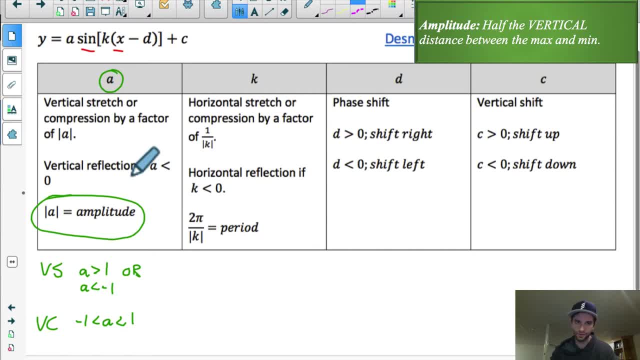 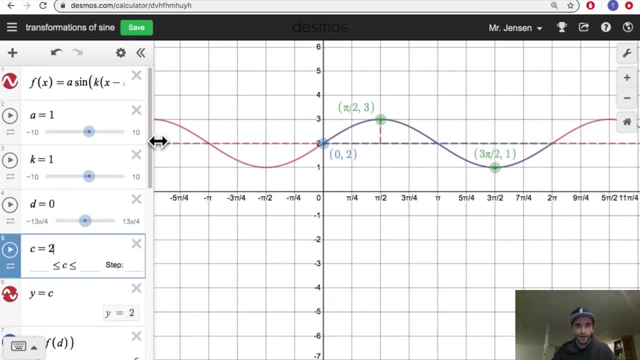 between the midline of the function and the max, or from the midline of the function to the min. So let's take a look at this. Let me reset it, Let me actually shift it up a little bit so we can see the function drawn in. And the amplitude of a function is the distance from the midline to the 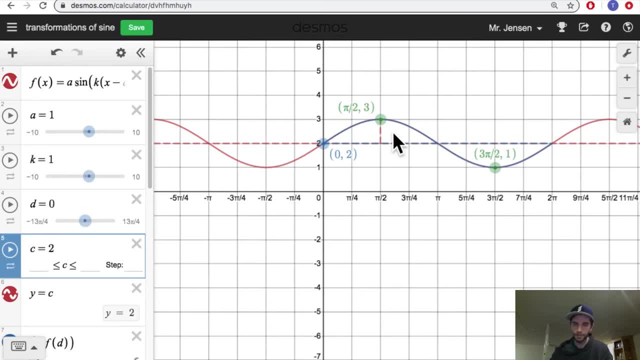 max. right, That's half the distance between max and min. That's amplitude. So for this function, what's the amplitude? Well, the distance from the midline to the max is one unit. It's one. That's because the a value is one. What if I make a value two? What's the amplitude? What's the distance? 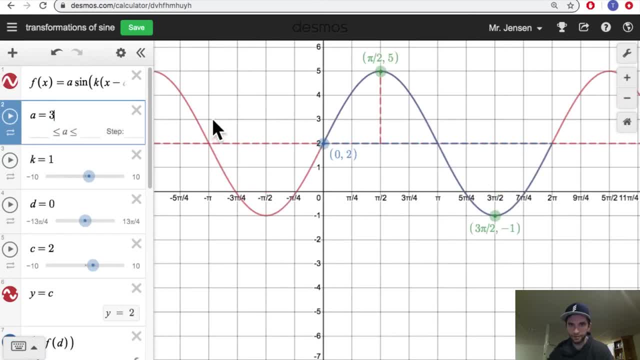 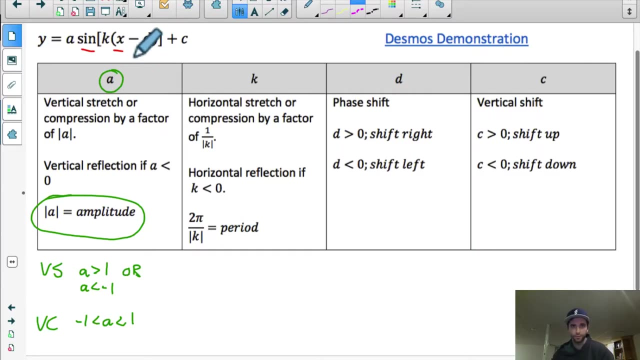 from midline to the max. It's one, two. I make a three. Amplitude is three. I think you get it. What if a is negative three? Well, the distance from the midline to a max point is still one, two, three. So the amplitude is the absolute value of a. Let's move on to the k parameter. 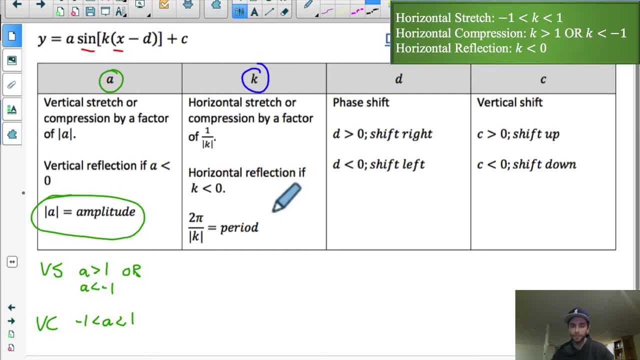 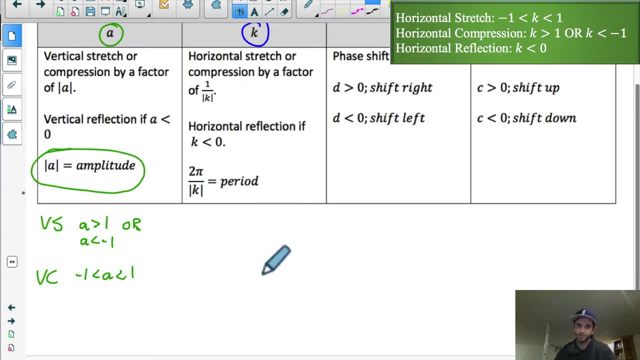 So a k parameter does a horizontal stretch or compression by a factor of the reciprocal of the k value, So by a factor of one over the absolute value of k. And if k is less than zero there's also a horizontal reflection. So these properties are in reverse of what it was for the 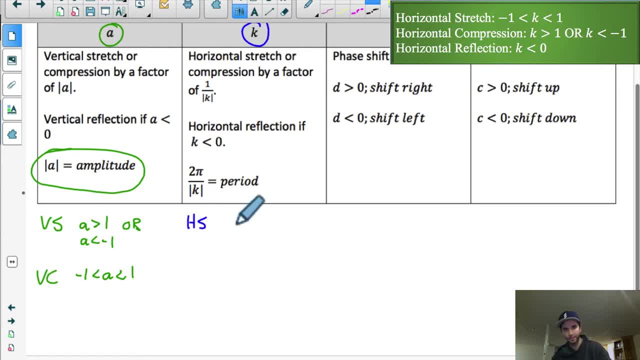 vertical stretch or compression. So there's a horizontal stretch If k is between negative one and one, And there's a horizontal compression if k is bigger than one or if k is less than negative one, And let me show you that in Desmos as well. So let me reset this function. 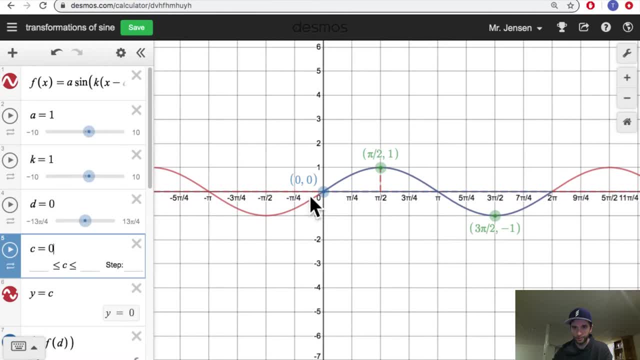 again. So I have one cycle mapped off for you in blue here. So here's one cycle, the function right, It takes two pi radians to complete one full cycle for a sine function. If I make k bigger, So if I make k two, it actually does a. 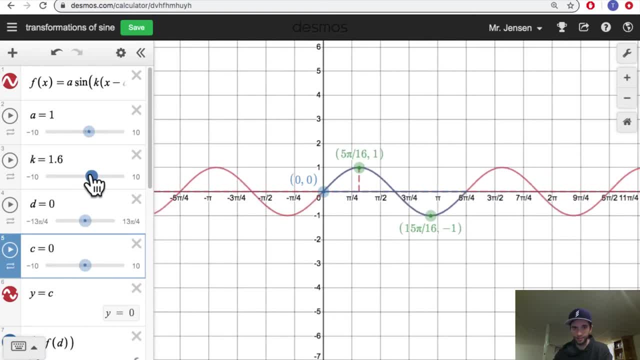 horizontal compression by a half. Look at how, look at the horizontal length of that cycle. when I make k two, The horizontal length of that cycle is half of what it used to be. It's no longer two pi, It's only pi, And I have that mapped off in blue here for you. So k does a horizontal. 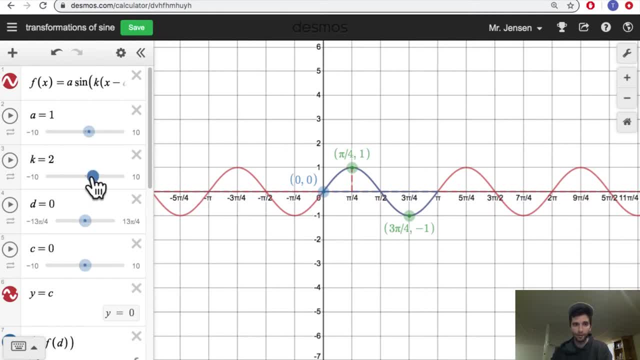 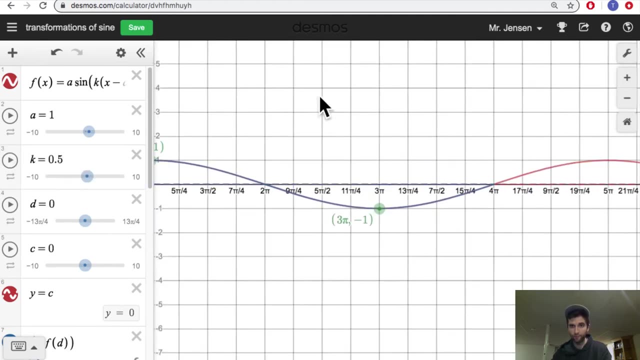 compression by one over two. in that scenario, How would I horizontally stretch it? If I made k a half, Let me put it to a half. Notice that's a horizontal stretch by a factor of two Instead of a half. I'm going to put it to a half. So I'm going to put it to a half. So k does a horizontal. 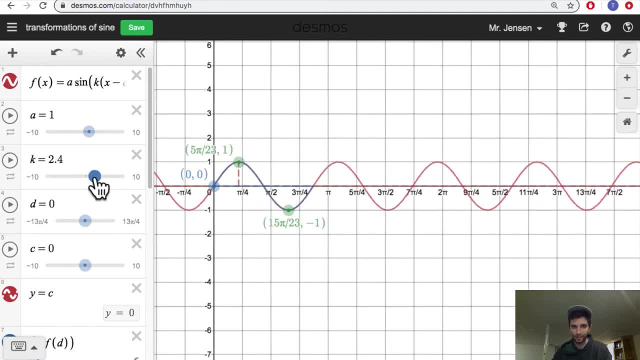 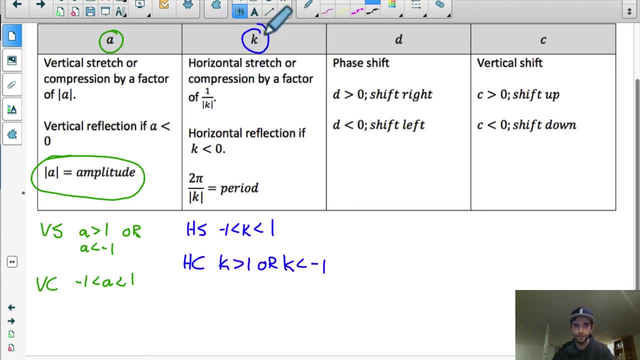 stretching and compressing. Horizontal stretching and compressing is what the k does, And if k was negative, it also does a horizontal reflection. So that's all summarized in the table right here. The k value does a horizontal stretch or compression by a factor of one over the 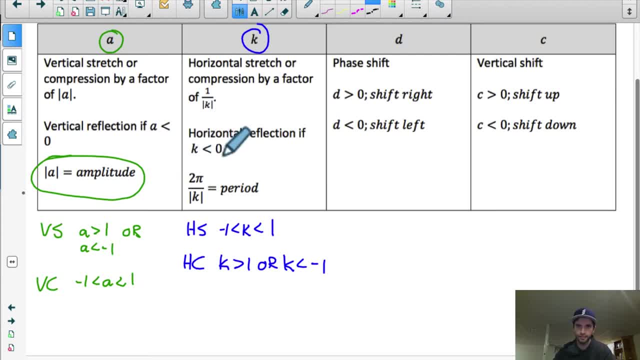 absolute value of k and it does a horizontal reflection if k is less than zero. So let's say k was negative three, We would say that there was a horizontal compression by a factor of three, But we would also say there's a horizontal reflection because that value is. 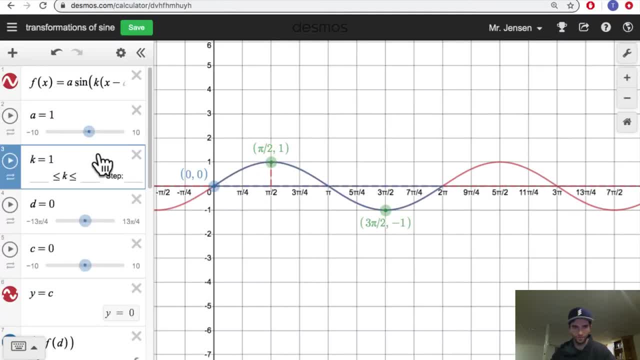 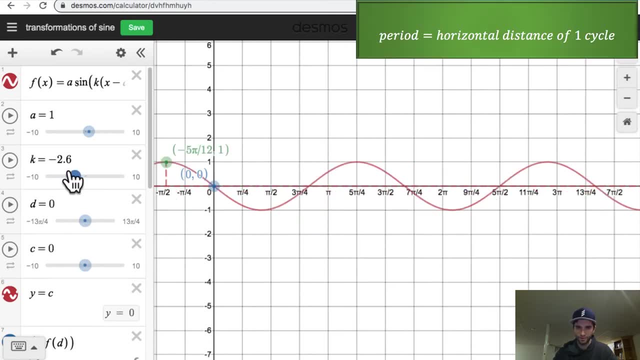 negative And I was trying to indicate to you in this Desmos graph that by manipulating the k value we see that the period of the function is also changing. So because it does a horizontal stretch or compression, that impacts the period of the function And we can calculate the new period. 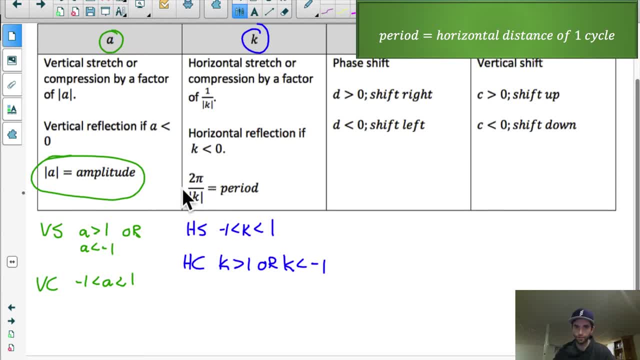 of the function by taking the period of an original untransformed sine or cos function- two pi- and multiplying it by one over k, Or another way of writing that two pi divided by the absolute period of the transformed function. Let's move on to the easier two transformations. 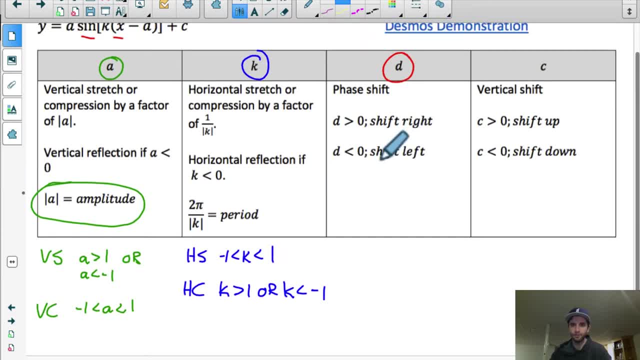 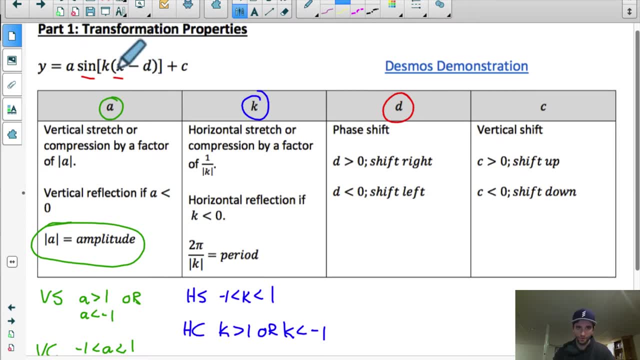 The d value just shifts the function left or right. So if d is positive it moves it right, If d is negative it moves it left. But keep in mind that the general format of a transformed function is x minus d. So if the d value is positive, let's say the d value. 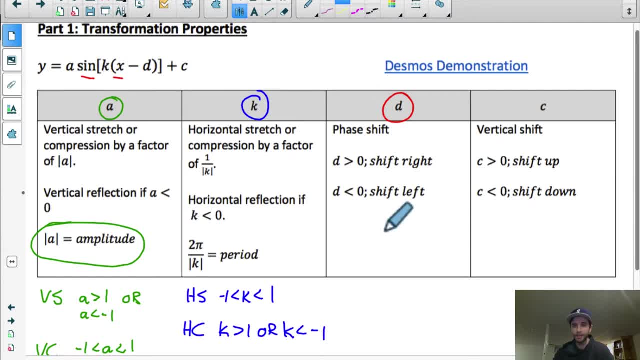 is five, It would appear in the equation as x minus five. And if the d value is negative, like, let's say, the d value is negative three, It would be x minus negative three. So it appear in the equation as x plus 3.. so a positive d value shifts it right. a negative d value shifts. 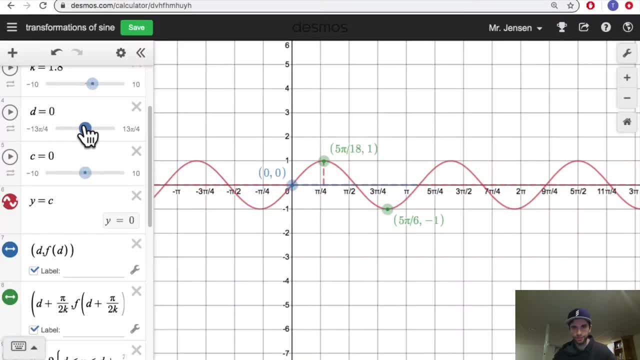 it left, but in the equation it'll appear as the opposite sign. so let me show that to you in desmo. so let me manipulate the d value. as i make the d value bigger, it moves it right. if i make the d value negative, it moves it left. so the d value just shifts it left and right. and lastly, let's 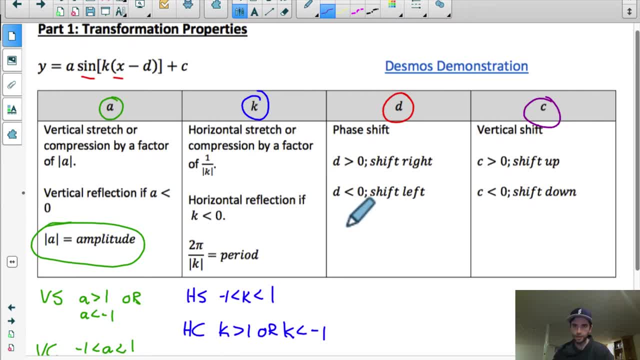 look at the c value. so the c value shifts the function up or down. so if c is positive, shifts it up, c is negative, shifts it down. and another thing that i want you to know is the c value tells you the horizontal midline of the function. so if we know the c value, we know where the 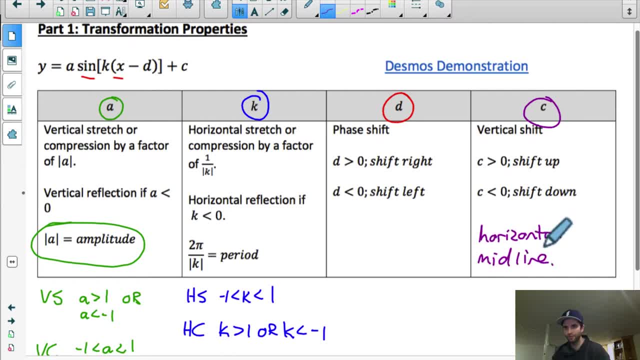 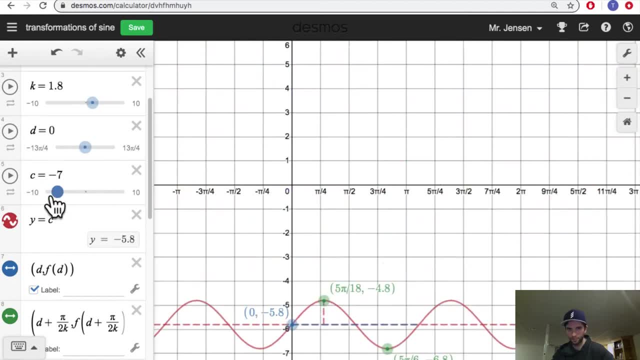 horizontal midline of the function is, and that's going to be, an important property of sine and cosine functions. so as i manipulate the c value, right, if i make c bigger it moves it up, if it makes you smaller, moves it down. but notice, the c value matches where the horizontal midline is. 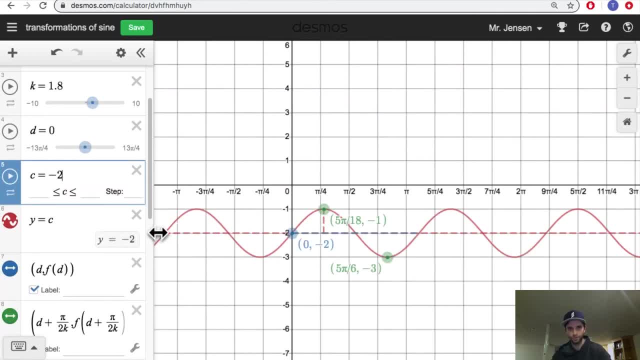 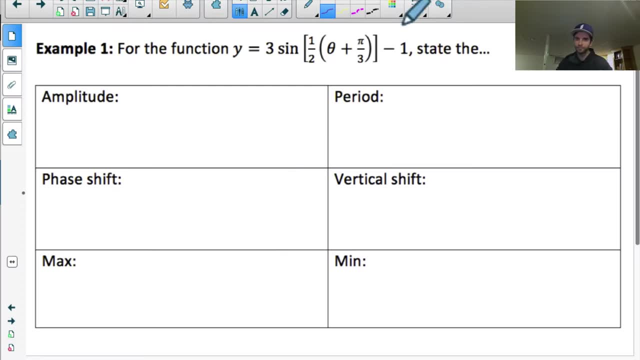 if i make c negative 2, notice there's a horizontal midline at negative 2 through that sine function. so let's actually go ahead now and let's fill out some properties of this function, now that we understand what the parameters a, k, d and c do to transform a function. 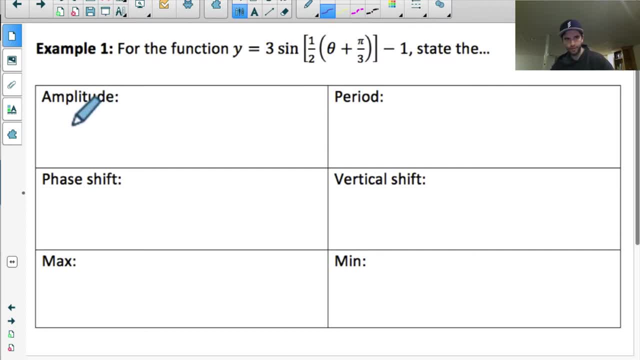 so the amplitude of this sine function- hopefully remember the amplitude- is equal to the absolute value of a. so in this case, here's the a value. so the absolute value of 3 is just 3.. the period of the function we can calculate by doing 2: pi. 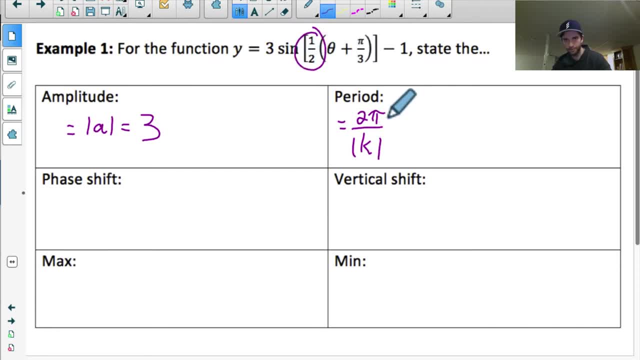 divided by the absolute value of k, and in this case the k value is a half. so we do 2 pi divided by a half. dividing fractions, flip and multiply. so 2 pi times 2 over 1. so 2 pi times 2 is 4 pi and this should make sense to you. the period is 4 pi because this would cause a horizontal. 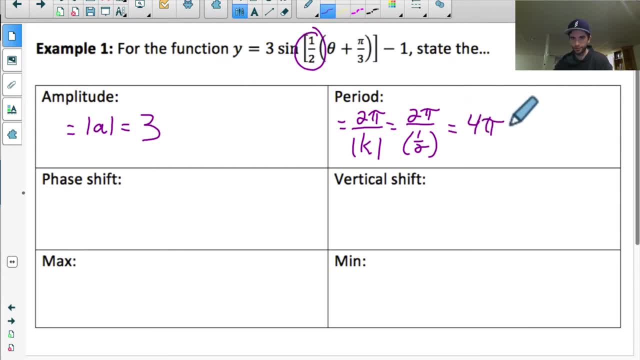 stretch by a factor of 2. so it's going to double the period of the function. phase shift. that means left or right. so the d value of the function is actually negative. pi over 3. so that means shift left. pi over 3 radians. vertical shift is negative. pi over 3 radians: vertical shift is negative. pi over 3 radians: 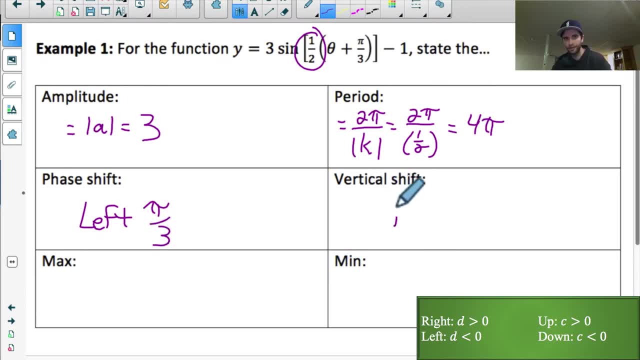 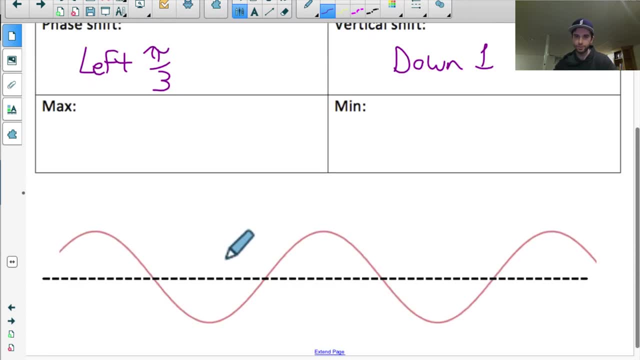 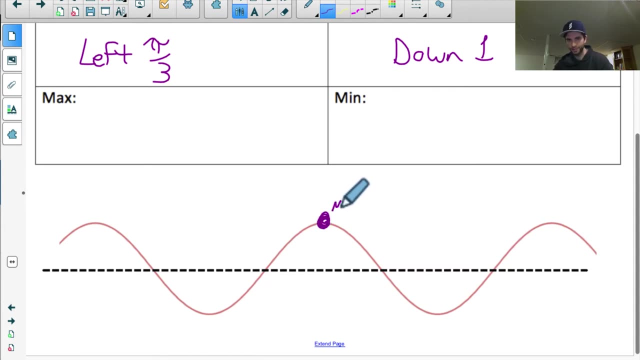 is based on the c value. the c value is negative. 1, that means move down one unit. if we want to calculate the max and the min value, let me just show you a diagram here, so i have a midline drawn in. if we want to figure out the maximum y value, a function ever gets to- 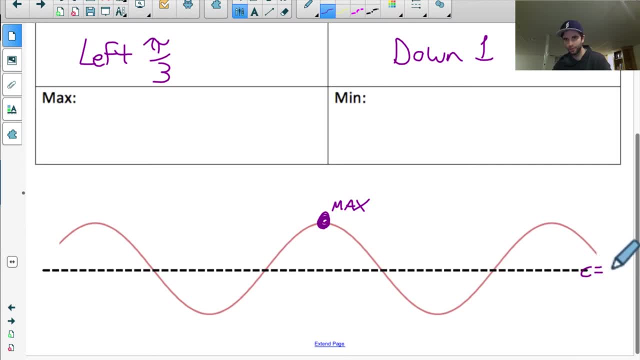 well, if we know the c value- and in this case the c value was negative one- i can figure out where the max is, because i know the distance between the midline and the max is equal to the absolute value of a. it's equal to the amplitude, and in this case the amplitude was 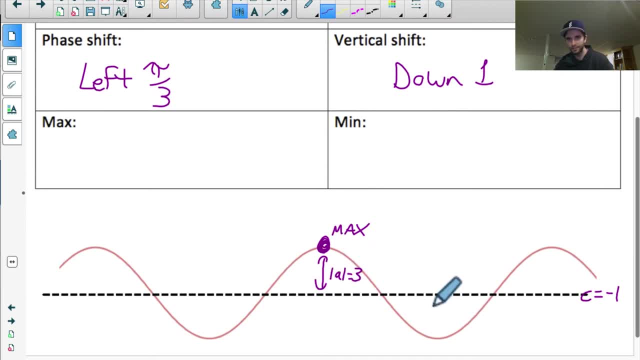 3.. so the distance between the midline and the max is 3, and the distance between the midline and the min is also equal to the absolute value of a 3.. so if i want to figure out the y value of this max, i just have to go to the middle of my function, so negative 1 and add the amplitude. 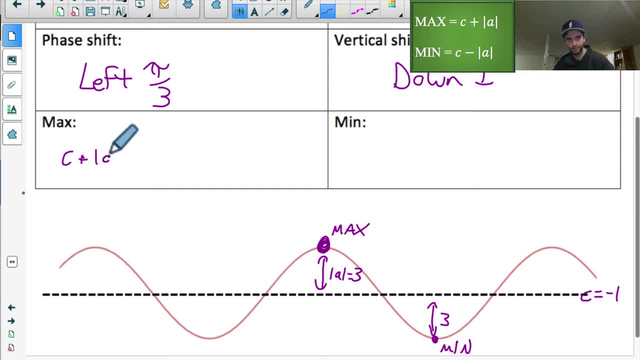 so add 3.. so just do c plus the absolute value of a, the y value of the max. so negative 1 plus 3 is 2.. the highest the function ever goes is to a y value of 2.. how about the min? well, you just go to the c value, the midline. 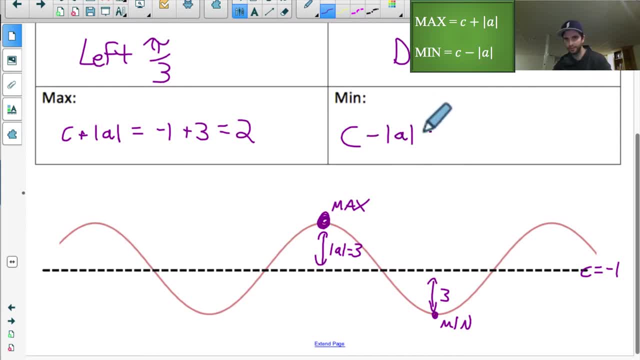 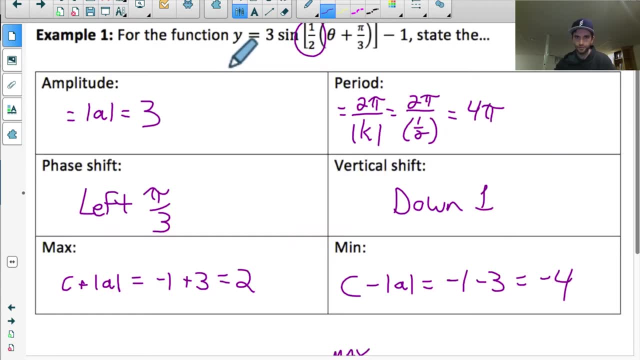 and then subtract the amplitude, so c minus the absolute value of a, so in this case negative 1 minus 3, that gives us negative 4.. so those are just some properties we could fill out about this function. now let's try a different equation and let's actually graph it this time. so let's graph. 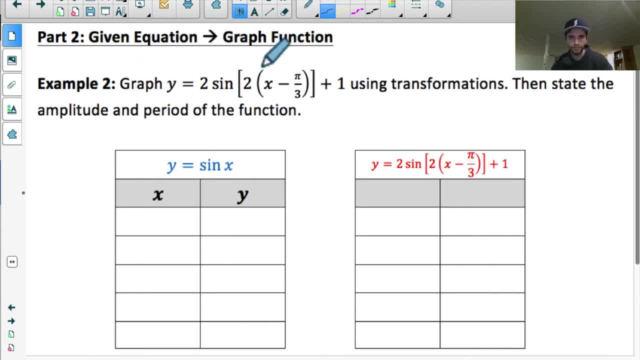 this transform sine function. we're going to do a different equation now. let's actually graph it this time. so let's graph this transform sine function. so this sine function is being transformed in four ways. here's our a, k, d and c parameters. if we're going to graph a transform sine function, it would be useful to generate a table of points. 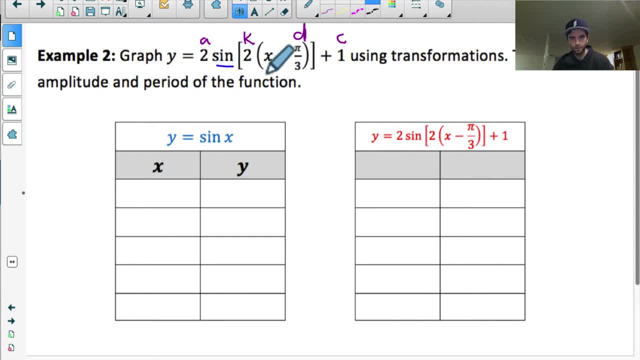 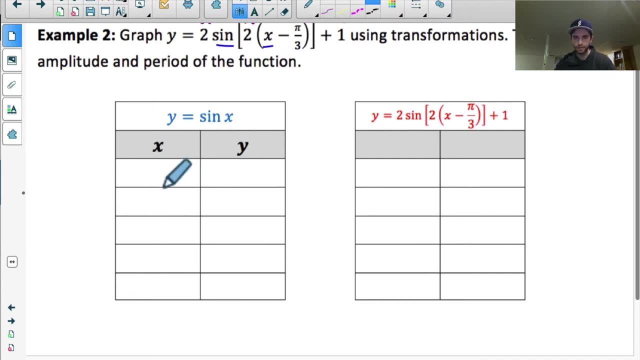 for the parent function. in this case the parent function is sine x because that's the function that's being transformed. so let's pick some x values for sine x. that will give us a good picture of one cycle of the function. well, sine x before it's being transformed. 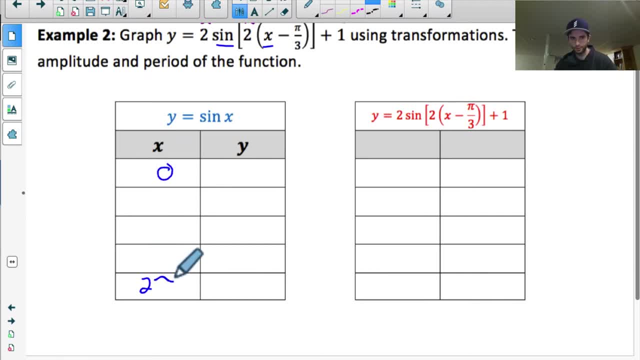 has a period of 2 pi. so i need x values between 0 and 2 pi and i think going up by pi over 2 will give us enough points to give us a good shape of that cycle. so 0 pi over 2, 1 pi over 2, 2 pi over 2. 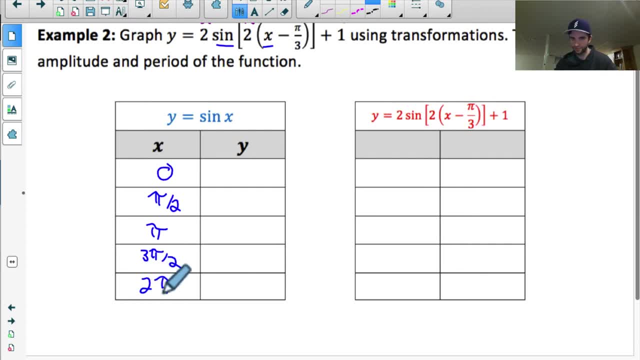 3 pi over 2 and finish at 4 pi over 2, which is 2 pi. now let's calculate the y values by evaluating sine of each of those angles right. take each of those, plug them in for x and if you know your unit circle well, you should be able to generate these relatively quickly. i know sine and. 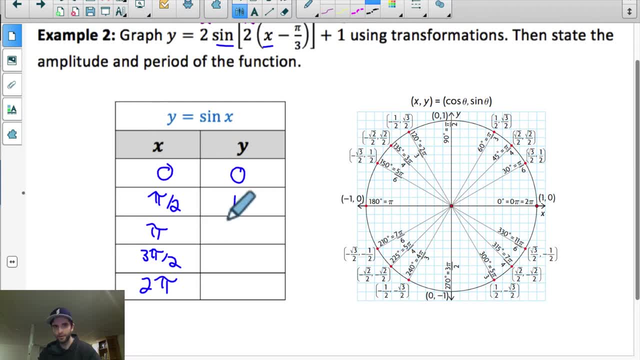 0 is 0, sine of pi over 2 is 1, sine of pi is 0 sine, and 3 pi over 2 is negative 1 and sine of 2 pi, all the way back to where we started at 0.. so here are 5 points that would give us a. 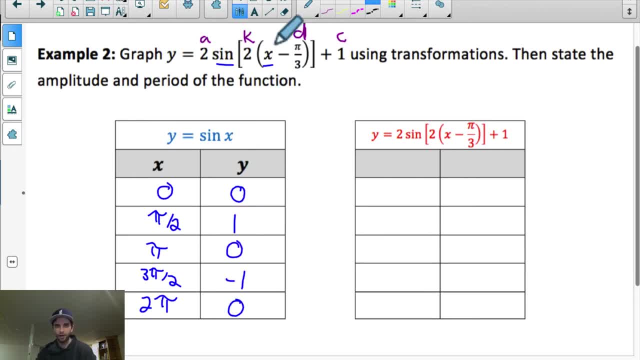 good shape of the sine function. but what we want are points for this transform sine function. so we have to perform the transformations to these points. and what transformations are happening? well, in this case there's a horizontal compression by 1 over 2, right? so i'm just going to. draw right only front and back. finish the определization if i want right content. so if i don't want to just add the point, so if i don't want to add the point, just fine and just end with the point. so much powerfo기에, and i'm just going to go over to anchor and just E and t and so on for the 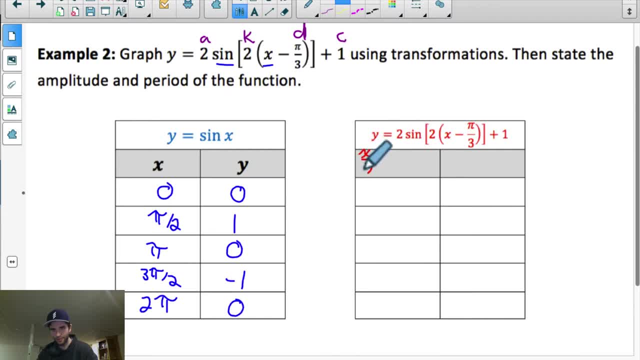 topave and just find all of your skeptical Teternal Architect. these frequencies any'll be換 right. so i have to take each of the x values and cut them in half and it's being shifted right- pi over three. right, the d value is pi over three, which means right, pi over three. so i'd have to. 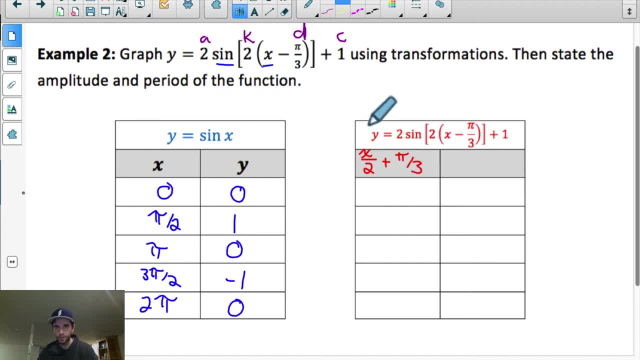 add pi over three to each of the x values. so the general, the general equation i could use to come up with what goes here is: we do x over k, right, that multiplies x by the reciprocal of k, and then we add whatever the d value is. now let's figure out what transformations are happening to the y. 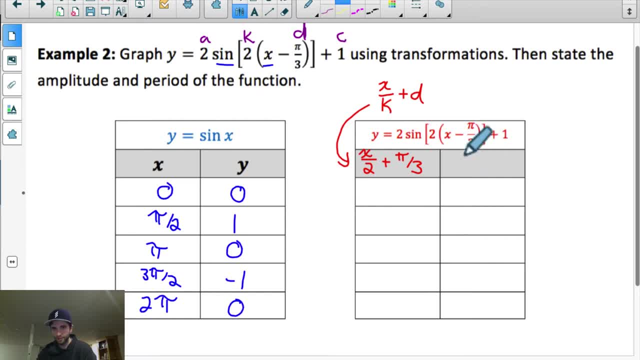 values. so the a value vertically stretches the what the function by two. so we'd have to multiply all the y values by two. and the c value shifts the function up one, so i'd have to add one to all the y values. so the general equation i could use to come up with what goes here: 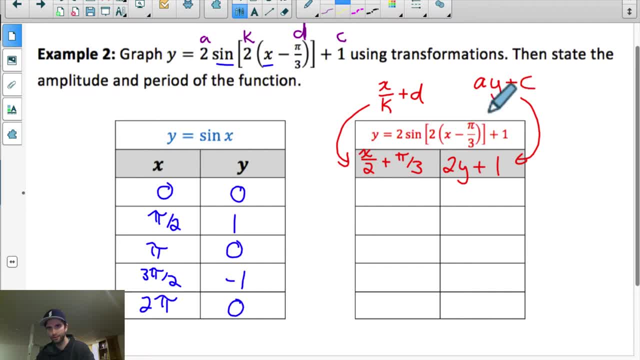 is a times the y value plus c. and then i'm going to use these equations i came up with to transform these x and y values to get x and y values for the transformed function. so take each of these x values, plug them in for the x into this little equation we made. 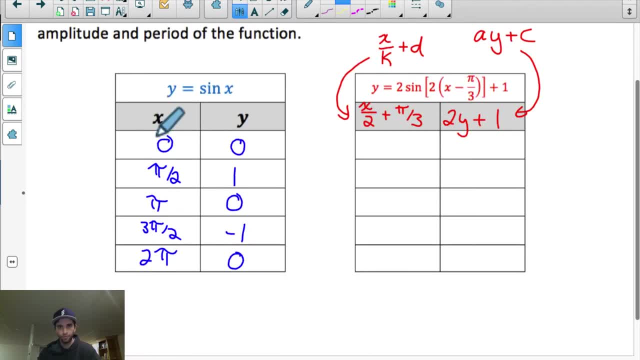 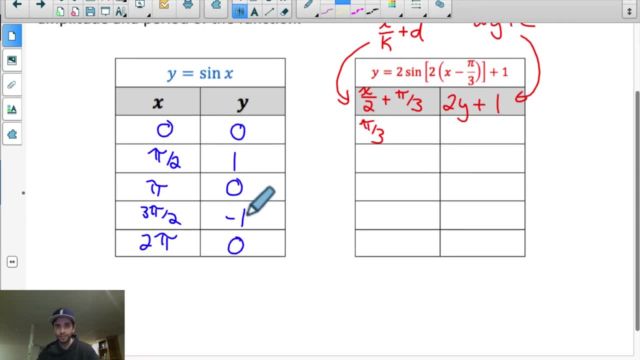 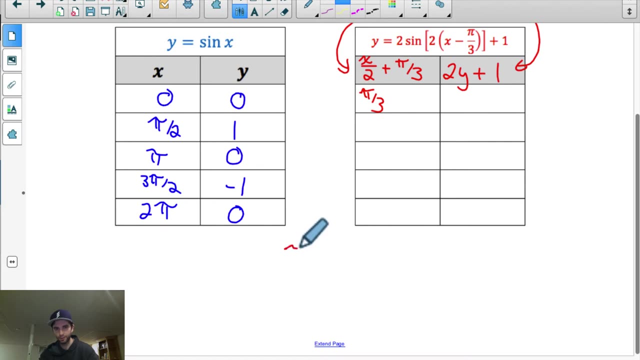 and we get the transformed x values. so plug zero in, that's easy. zero over two is zero, plus pi over three is pi over three. the next ones are going to be a little more difficult because we're going to have to do some fraction work. so if i plug pi over two in for x, i'll do the work down here. i'd have 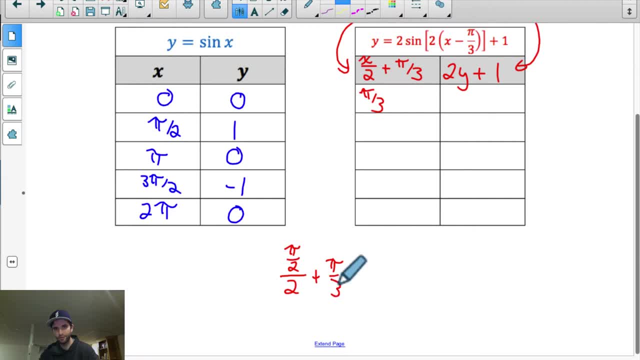 pi over two over two, you plus pi over 3. well, pi over 2 over 2. flip and multiply, we get right. this is 2 over 1 here. flip and multiply, i get pi over 4. so i have pi over 4 plus pi over 3. adding fractions: i need a common 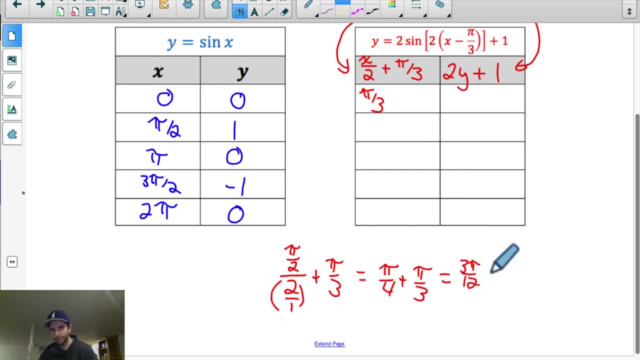 denominator. so it would be 3 pi over 12 plus 4 pi over 12, that's 7 pi over 12. so here, 7 pi over 12. let's do one more of these and i'll give you the last two. so 7 pi over 12. okay, so the third one. 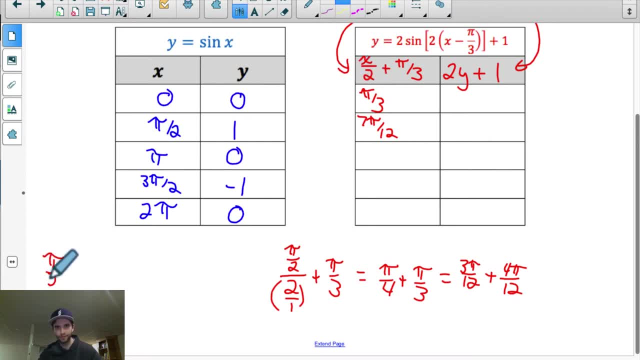 take this pi, plug it in here, so i'd have pi over 2 plus pi over 3. i would need a common denominator, so that would be 3 pi over 6 plus 2 pi over 6, that's 5 pi over 6. 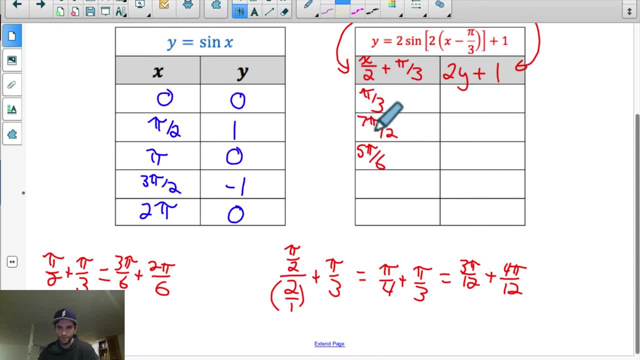 and now, if we look at the difference between these values, we should be able to use our patterning skills and come up with the next two. this is over 12, so i think of each of these is over 12, 4 pi over 12, 7 pi over 12, 10 pi over 12. the difference is: 3 pi over 12, so i think of each of these is over 12. 4 pi over 12, 7 pi over 12, 10 pi over 12. the difference is 3 pi over 12, so i think of each of these is over 12. 4 pi over 12, 7 pi over 12, 10 pi over 12. the 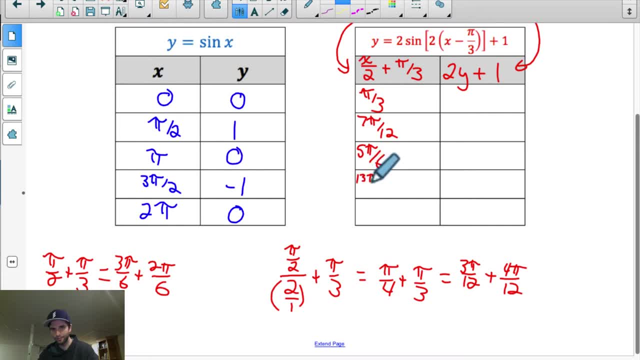 3 pi over 12 each time. So the next one will be 13 pi over 12, and after that will be 16 pi over 12, which reduces to 4 pi over 3.. So I have all my x values. Now I have to calculate the y values. 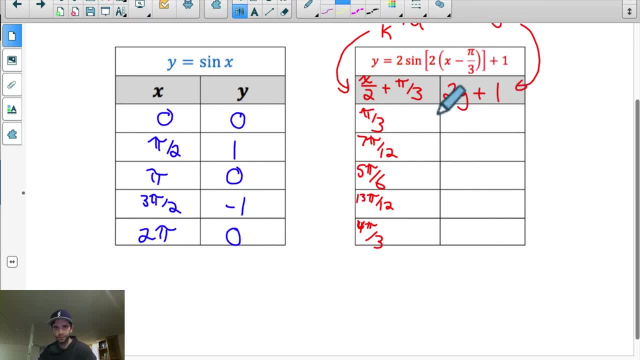 so take each of these y values, plug them into this little equation I made and I get the transformed y values. So plug 0 in 2 times 0 plus 1 is 1.. Plug 1 in 2 times 1 plus 1 is 3,. 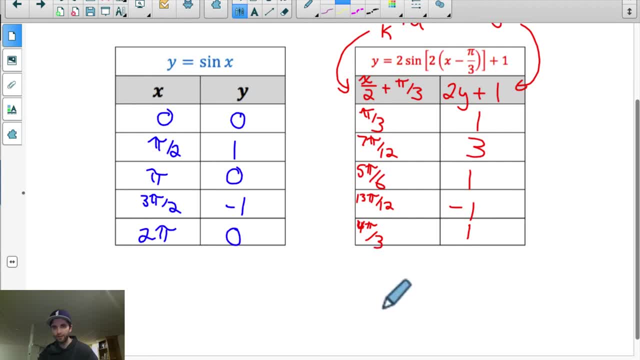 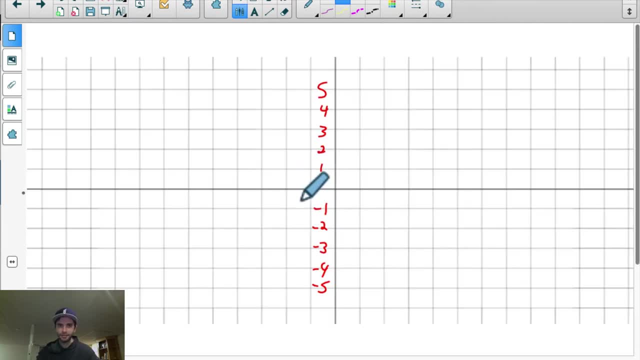 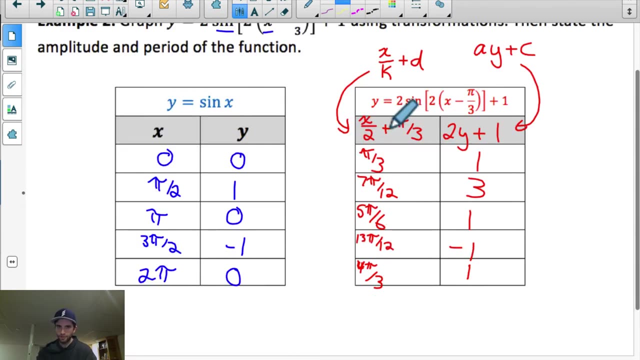 and so on. Now that I have my points, I need to graph them, but it's a little more difficult than usual because I need to carefully choose my scales. So on the y-axis, I decide to make my scale just go up by 1s. but for the x-axis we have to very carefully choose a scale. Some of 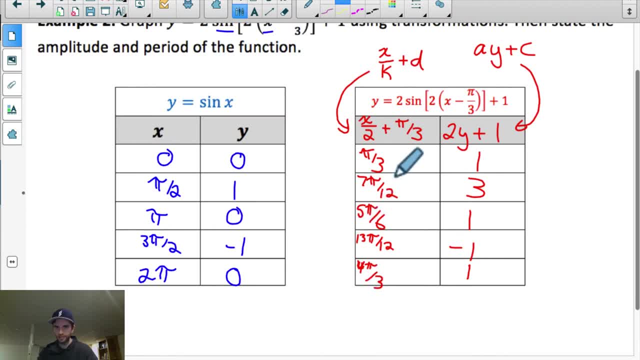 my fractions here are over 3,. I have an over 6 fraction, I have 2 over 12 fractions. So let's say, let me just walk you through a thought process you might go through. Let's say you thought you might want to go up by pi over 12.. 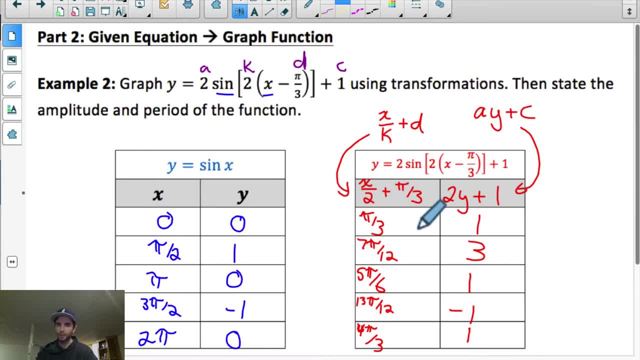 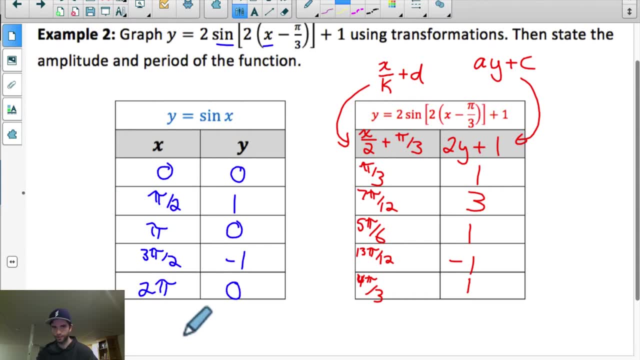 Oh, and I should mention, whenever we're graphing the transformed function, I'm always going to ask you to graph two cycles of the transformed function. So this is one cycle, right? because we transformed one cycle of sine x and we want to leave room to be able to graph an entire another cycle as well. 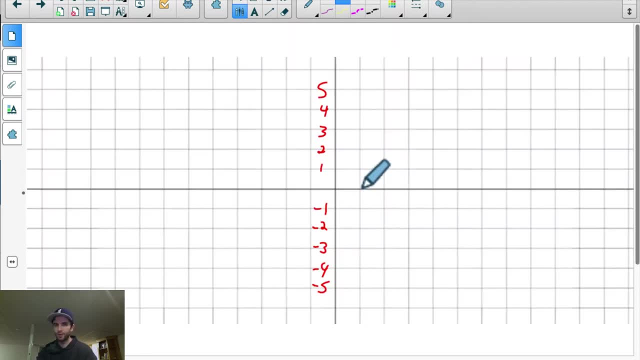 So let's say you thought you might want to go up by pi over 12.. If you went up by pi over 12 on the x-axis, this would be 1 pi over 12,, 2 pi over 12,, 3 pi over 12, and so on 4,, 5,, 6,, 7,, 8,, 9,. 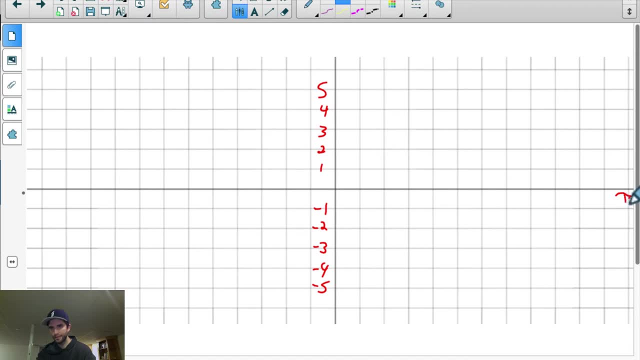 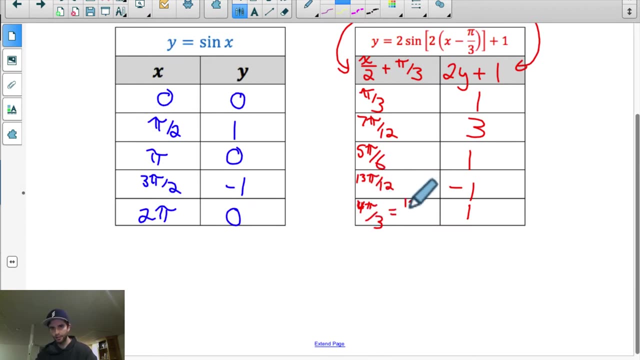 10,, 11,, 12.. Here would be pi, because that would be 12 pi over 12.. And this last point here, if we're over 12, would be 16 pi over 12.. So that point wouldn't even fit on this graph. 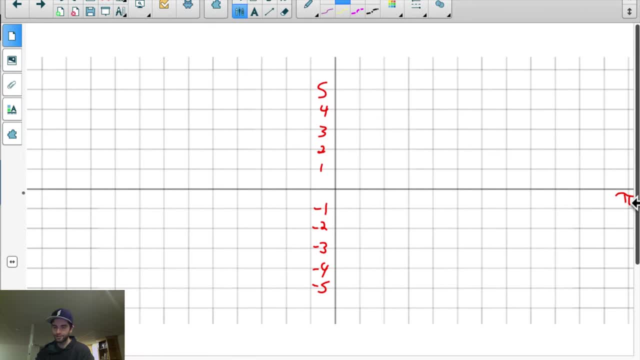 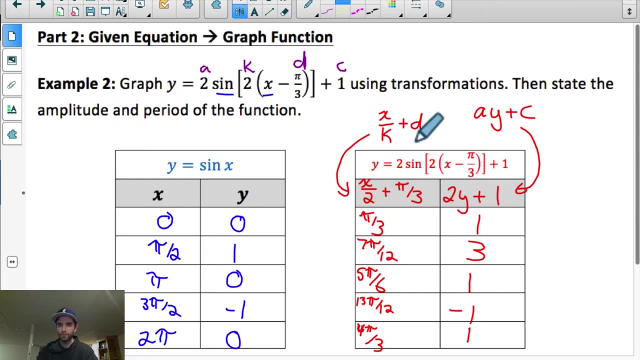 right, I don't have 16 units to the right of the y-axis, So going up by pi over 12 is not going to work. So how about pi over 6?? What if we went up by pi over 6?? If I went up by pi over 6, I would. be able to graph a whole cycle of sine x and so on. So let's say you thought you wanted to go up by pi over 12, and so on. So let's say you thought you wanted to graph a whole cycle of sine x and so on. So let's. 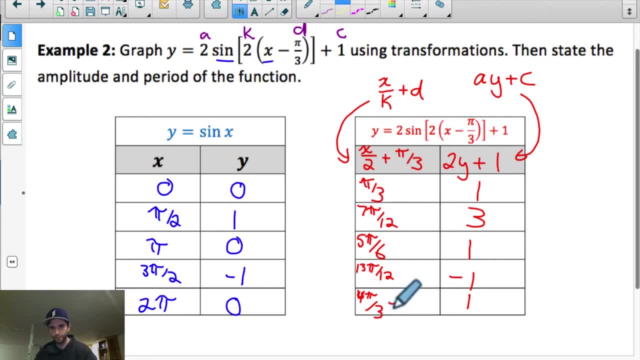 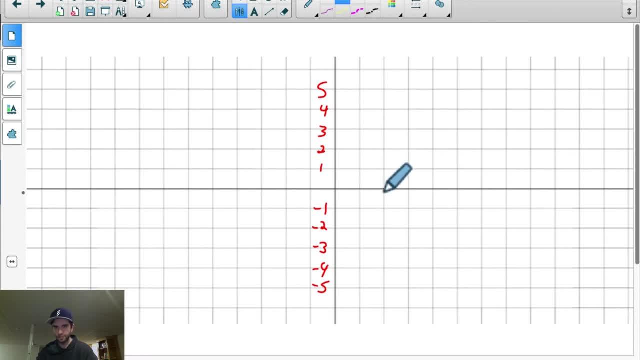 pi over 6, that would mean that this one was 8 pi over 6.. Would that fit on the graph? So if I went up by pi over 6, this would be 1 pi over 6,, 2 pi over 6,, 3 pi over 6,, 4, 5, 6 pi over 6.. So here: 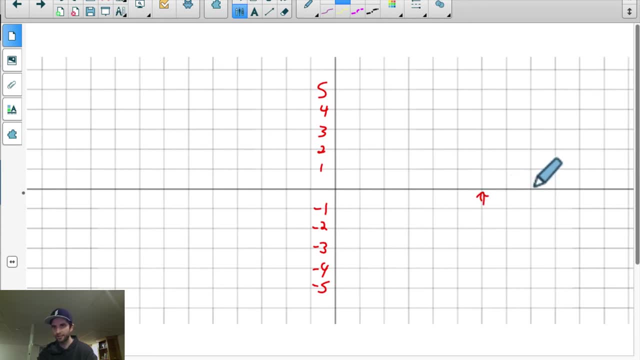 would be pi, 7, pi over 6,, 8 pi over 6.. Yes, so the point with an x value of 8 pi over 6, yes, would fit on the graph. It would be right here, and its y-coordinate is 1.. So the function would start at: 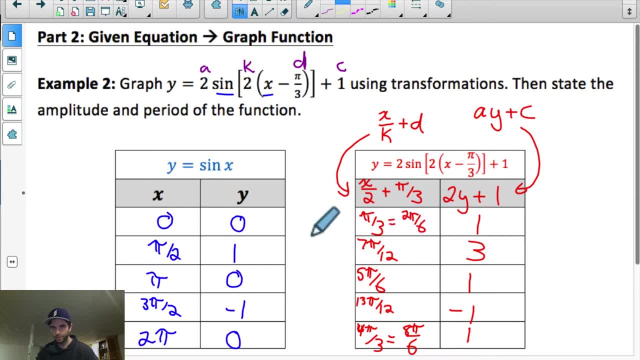 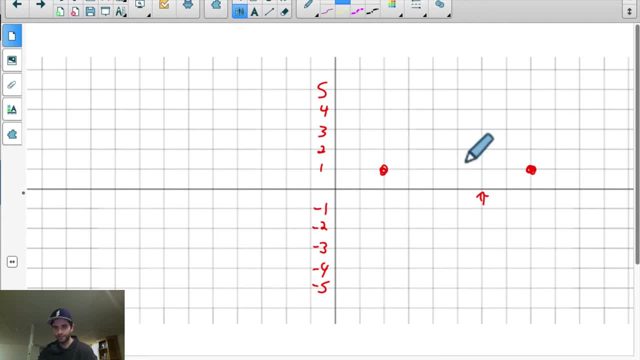 this is 2 pi over 6, so it would start at 1 pi over 6,, 2 pi over 6, y value of 1.. So it would start here and it would finish here. There's one cycle And then, yes, there's room over here to do another. 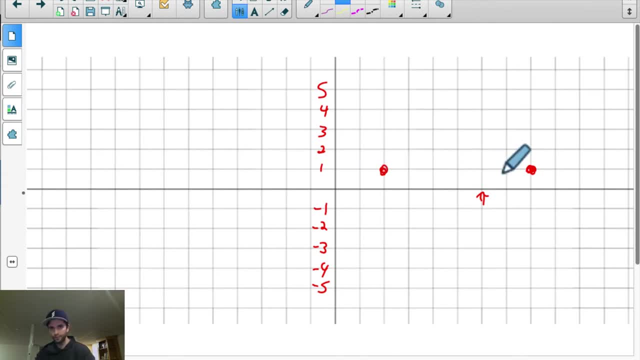 cycle. So notice it takes 1,, 2,, 3,, 4,, 5, 6 pi over 6 to complete one cycle. So 1, 2,, 3, 4, let me count again. So 1,, 2,, 3,, 4,, 5, 6.. It'll complete the other cycle. 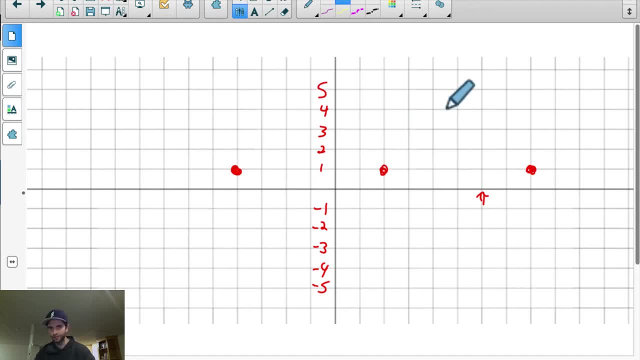 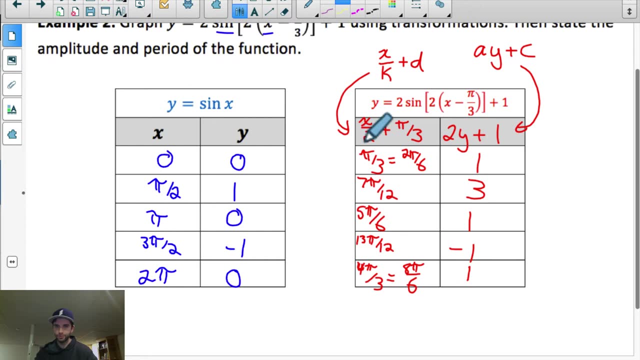 by the time it gets to here. So I'll be able to get two full cycles in between here. So if I'm going up by pi over 6, it's going to be useful to rewrite each of these fractions as fractions with a denominator of 6.. That way the numerator tells me how many tick marks I need to. 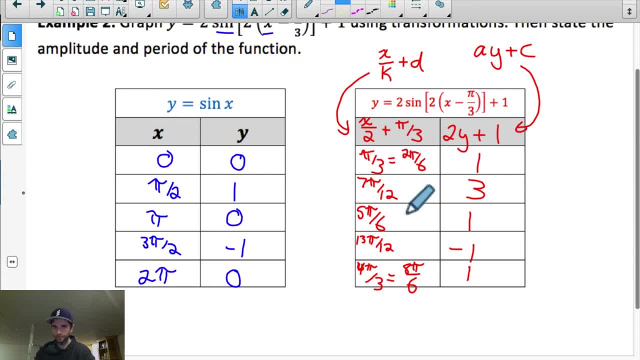 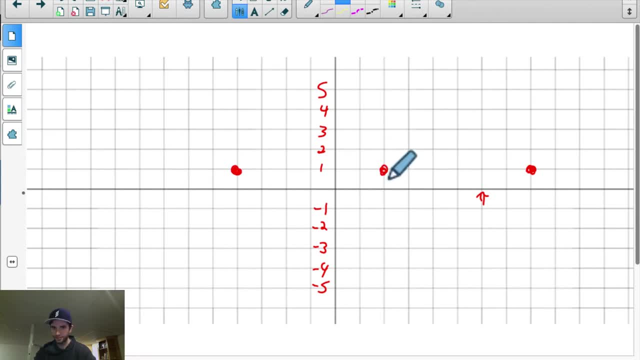 move over when graphing it. So notice, when I graphed this point, 2 pi over 6 comma 1, since my scale is going up by pi over 6s, that means I go 1,, 2 pi over 6, and y-coordinate. 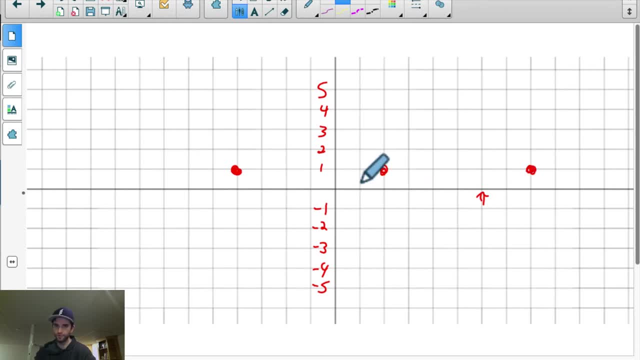 of 1.. When I graphed this point it was 8 pi over 6 comma 1.. So I move 8 tick marks 1,, 2,, 3,, 4,, 5,, 6,, 7,, 8 pi over 6, y-coordinate of 1.. And if you were looking at this graph you should easily be. 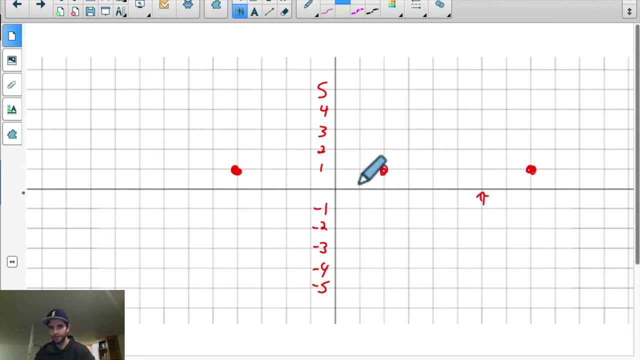 able to tell what the scale is. Just look for where's pi. Pi is at the 1,, 2,, 3,, 4,, 5, 6th tick mark. That must mean you're going up by 1 pi over 6, because this would be 6 pi over 6,, which is 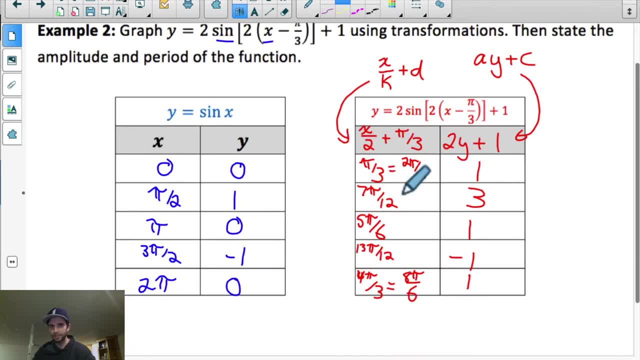 just pi. So let's plot the other points that we have by changing these to these two here to being over 6 fractions. So I would have to divide the top and bottom by 2 to make this be over 6.. So this would be 3.5 pi over 6. This one's already over 6.. Divide this one top and 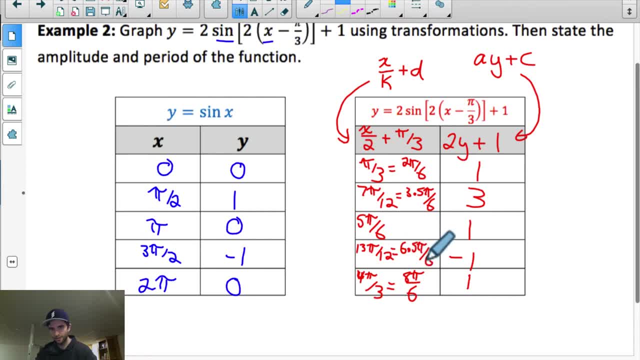 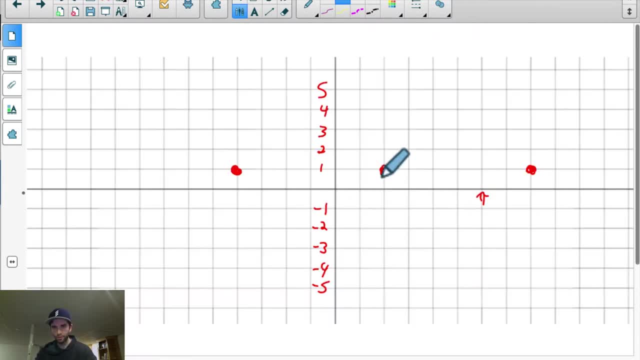 bottom by 2, and I get 6.5 pi over 6.. So let's graph the three points in the middle, So 3.5 pi over 6 comma 3.. That means go 1,, 2,, 3 and a half units and then 1,, 2,, 3.. 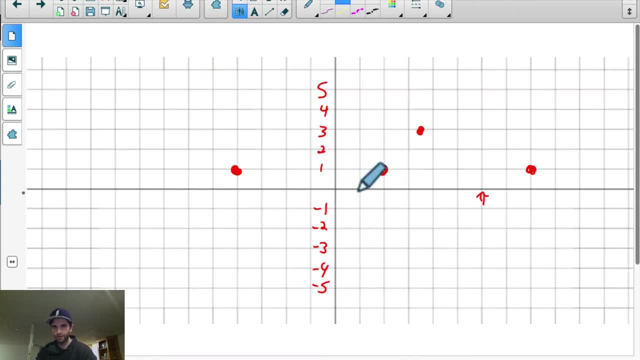 And then the next point was at 5 pi over 6 comma 1.. So move 5 units: 1,, 2,, 3,, 4,, 5,, 1.. And then the last one was at 6.5 pi over 6 negative 1.. So 1,, 2,, 3,, 4,, 5,, 6 and a half y-coordinate of 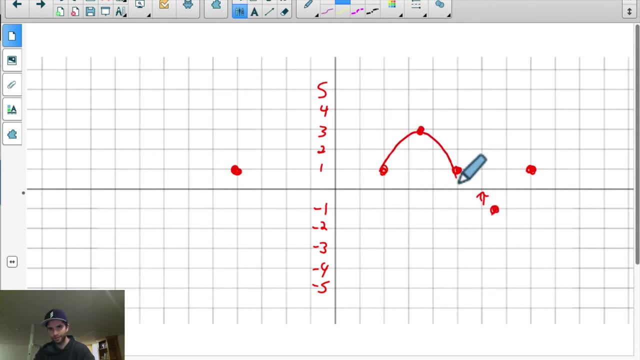 negative 1.. So here is one cycle of the function. Let's continue our pattern and do another cycle, And I should label some more points along the x-axis here, So the scale is more clear for you. right, We're going up by pi over 6.. So 1 pi over 6,, 2 pi over 6,, 3 pi over 6,. 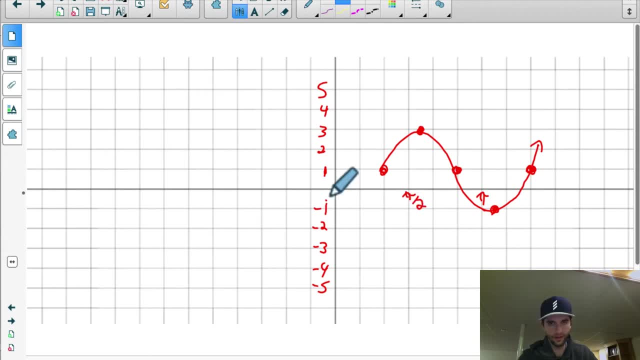 that's pi over 2.. And let's do some in the negative x-axis as well. So negative 1 pi over 6, 2, negative 3 pi over 6,, that's negative pi over 2.. And the sixth spot: 1,, 2,, 3,, 4,, 5, 6 will be negative. 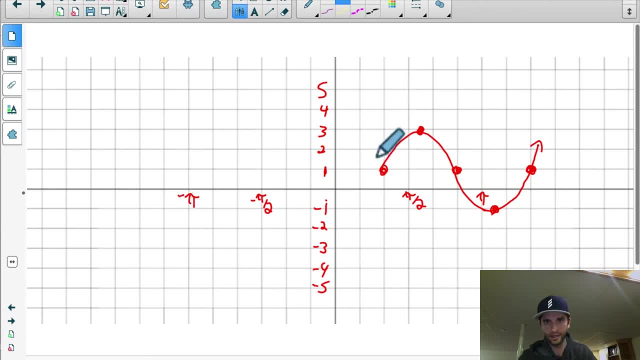 6 pi over 6, which is negative pi. Okay, let me do the other cycle now. I'll do it in a different color so you can more clearly see the difference between the two cycles. So it's periodic, right? So this cycle is just going to repeat over and. 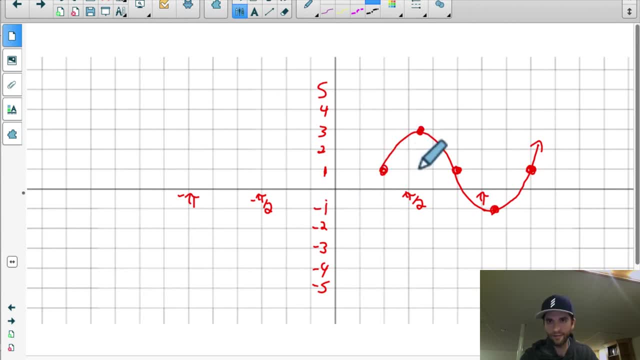 over again And notice there is a point. every one and a half units horizontally right Move one and a half to the right, there's a point, One and a half to the right, there's a point, and so on. So if I move one and a half to the left there'll be another point on my function. And if I follow, 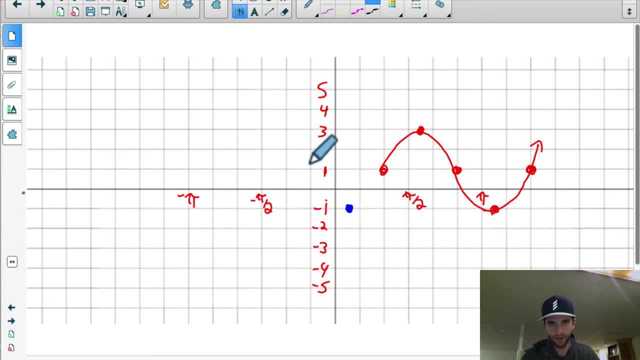 the pattern, it'll be down here. Move one and a half to the left, it'll be back up to here. One and a half to the left, it'll be up to here, And one and a half to the left. I'll finish my second. 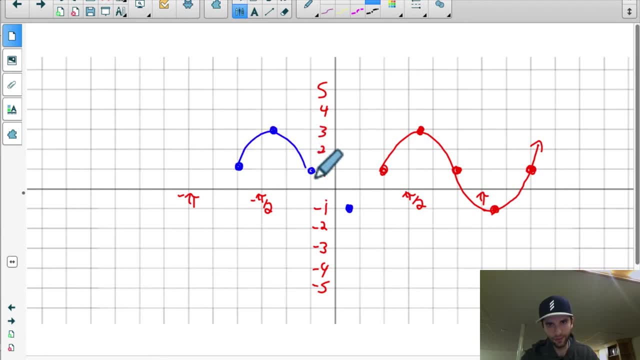 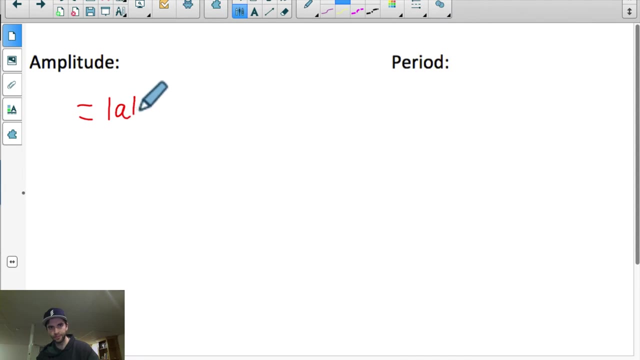 cycle right here. Notice that this cycle in blue matches the cycle in red exactly. So there's two cycles of the transform sine function. Let's write some properties of this function And if we have the equation of the function, the easiest way to find the amplitude is just do the absolute value. 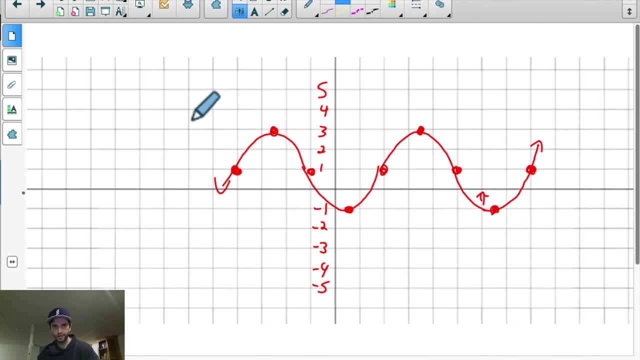 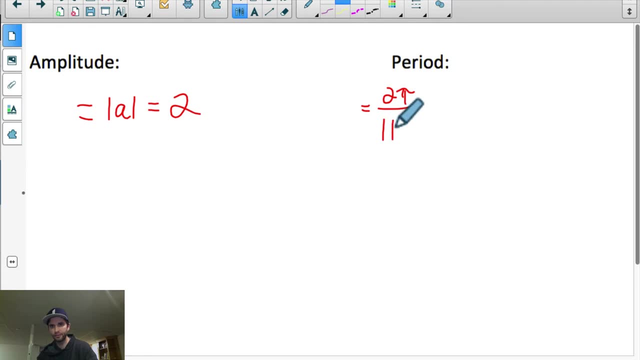 of a. So for this function the absolute value of a was 2.. So the amplitude is 2.. The period of the function is equal to 2 pi over the absolute value of k, And for this function the k value is 2.. So it's 2 pi over 2, which is pi right. So amplitude is. 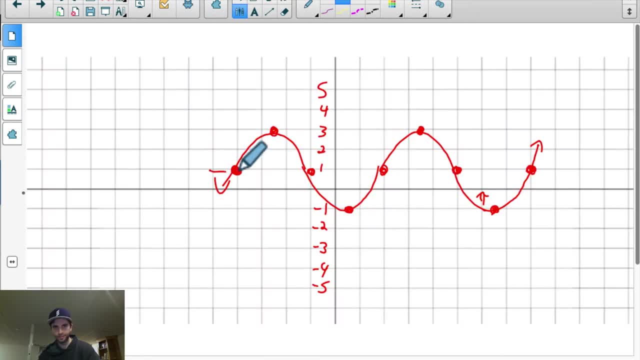 half the distance from max to min. Or another way of thinking about it is the distance from the mid line to the max. And yes, that distance is 2.. And the period of the function is the horizontal length of one cycle, And apparently that's pi. If I were to map off one cycle, here's one cycle. 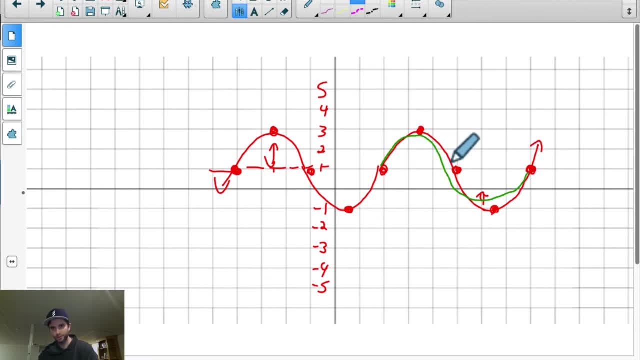 right here. The length of that cycle is 1,, 2,, 3,, 4,, 5,, 6,, 7,, 8,, 9,, 10,, 11,, 12,, 13,, 14,, 15,, 16,, 17,, 18,. 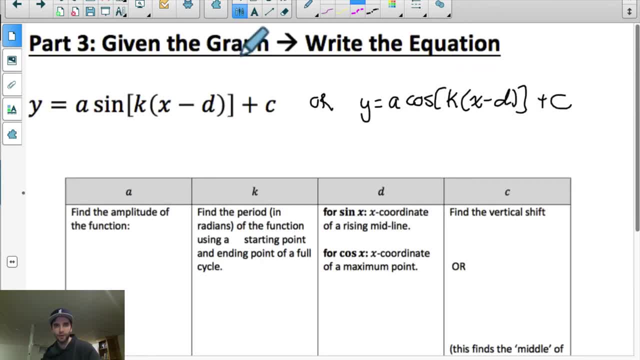 20,, 21,, 22.. So this is 1 pi over 6.. Now let's try where I give you the graph of the function And we figure out what transformations have happened to it and write the equation, And we should be. 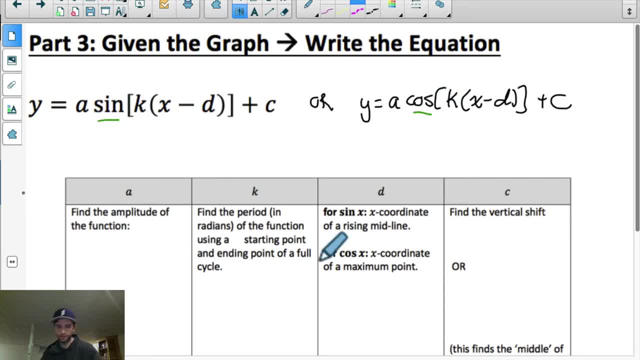 able to write a sine or a cosine function for any of these graphs. The only difference between the two of them is going to be the d value. Between a sine and a cosine function, the a, k and c values are going to be exactly the same, no matter which one of these two we are writing. The only thing. 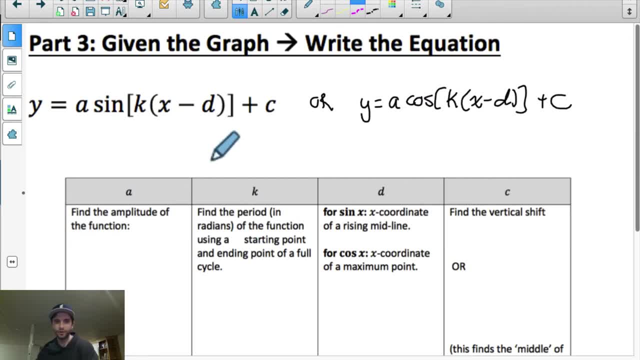 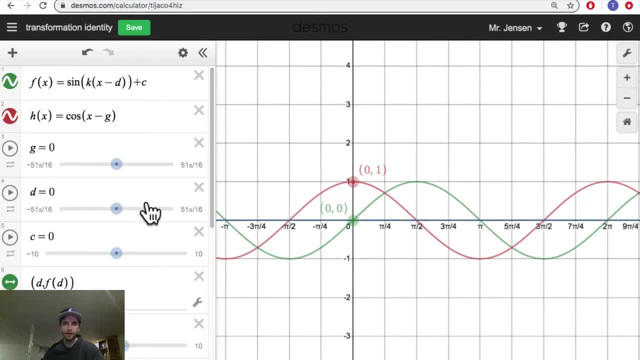 that will be different is the d value, the horizontal shift value. And then we're going to. Let me just quickly show you what I'm talking about in Desmos. So in red I have cos x, in green I have sin x. Now I don't have to describe this green function with the equation y equals sin x. 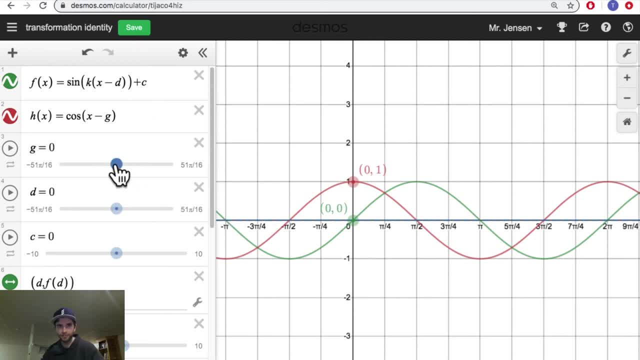 I could actually describe it with a cosine equation Because, watch, if I take this cosine function and shift it pi over 2 to the right, it overlaps exactly with that graph And same vice versa. If I wanted to describe this red function with an equation, 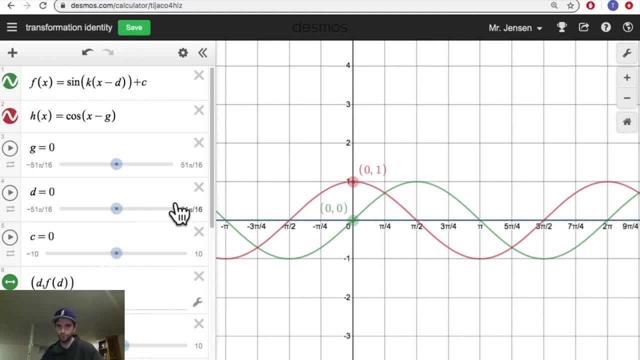 yeah, I could describe it with cos x, but I could also describe it with a transformed sine function, right? If I take the green sine function and shift it pi over 2 to the left, notice that it overlaps exactly with the cosine function. 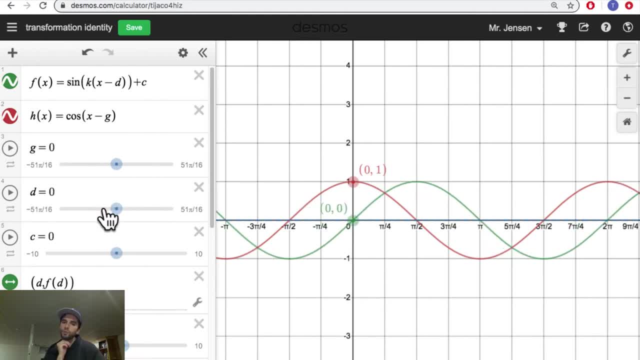 So this is just my way of showing you that we could write the equation of any of these sinusoidal functions with either a sine or a cosine equation, if we just manipulate the horizontal shift value accordingly. Okay, now let's talk about how we are going to calculate. 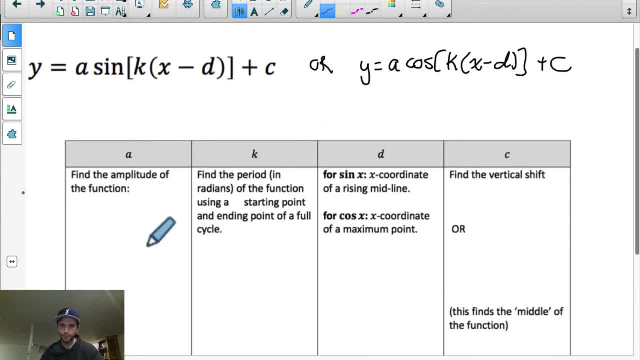 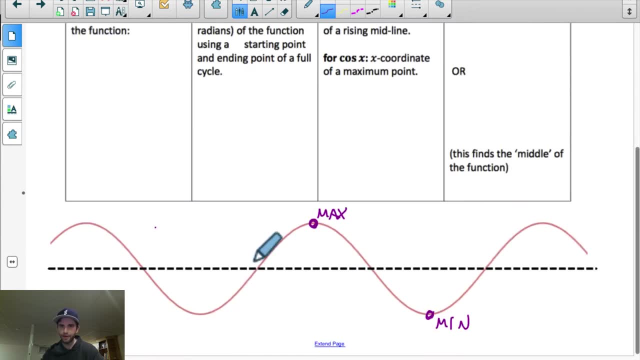 what these a, k, d and c parameters are by looking at the graph. So how are we going to figure out the a parameter? Remember, the a parameter is going to tell us the amplitude of the function. So how do we find the amplitude of a function? by looking at the graph. 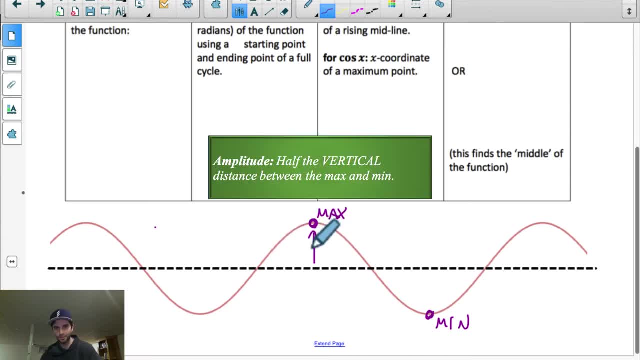 Well, we have to remember what the amplitude is. Amplitude is half the distance between max and min. So this would be the amplitude of the function represented by that line I drew there. It's half the distance between max and min. So the distance between the midline and the max. 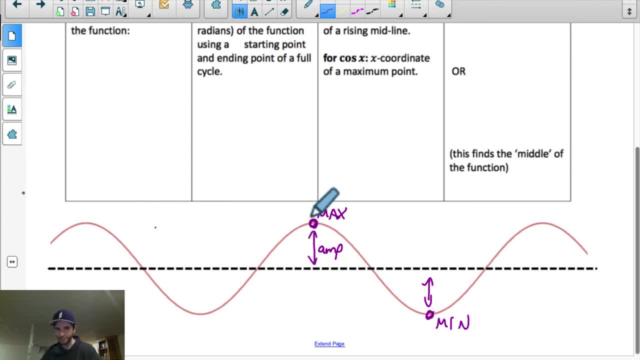 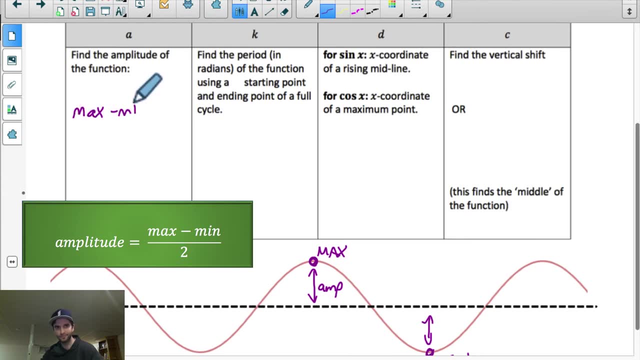 or from the midline to the min. That's the amplitude. So how do I find half the distance between these two points? Well, just find out what is the distance between the two points by doing max minus Min And then cutting it in half. 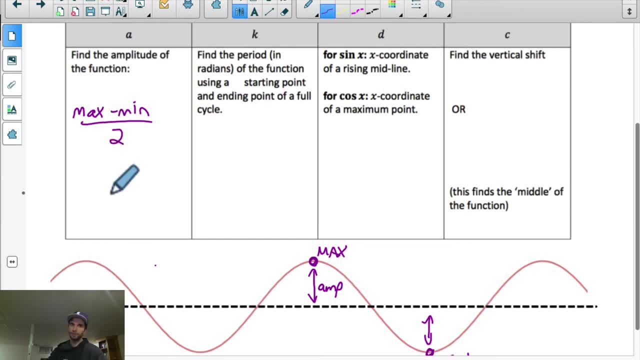 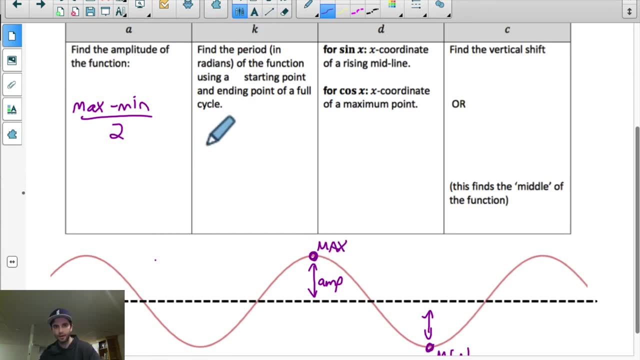 That's the amplitude. So we can calculate amplitude by doing max minus min over 2.. Next we're going to want to find the k parameter And if you remember before, remember the period of a function was equal to 2 pi over the absolute value of k. 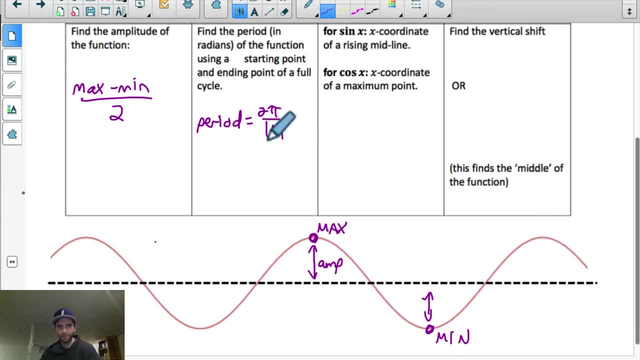 So we can manipulate this equation And notice that if we replace this k value with period, the k value equals 2 pi over period. right In algebra. if we rearrange that to isolate k, we get k equals 2 pi over the period. 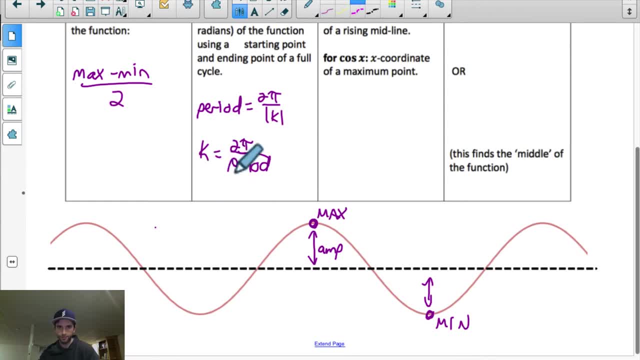 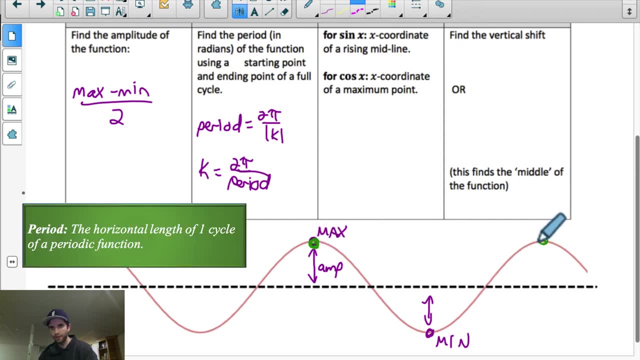 So how are we going to do that? by looking at the graph. Well, what's the period of a function? A period of a function is the horizontal distance of one cycle. So we just need to map off one cycle of a function. So we could. the easiest way to do that is probably between max points or between min points. 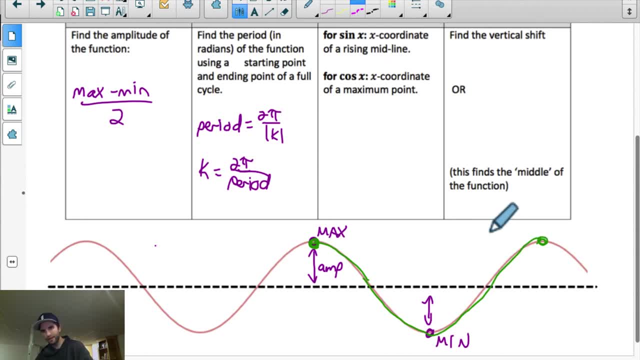 But we map off one complete cycle of the function And the horizontal length of that cycle. so from there to there, we call that the period of the function And we can calculate the k value by doing 2 pi over whatever the period is. 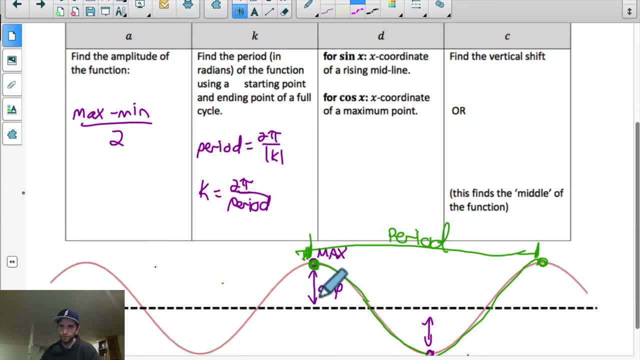 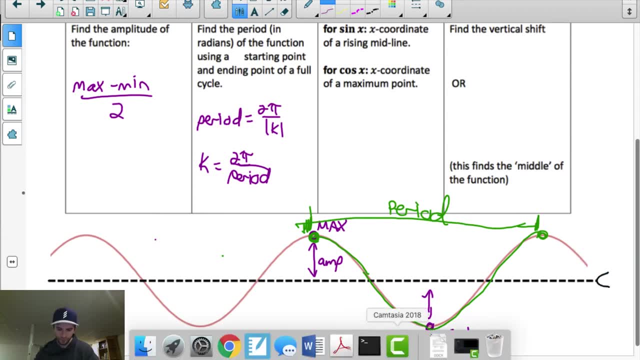 Let's skip d for now. I'll come back to that. Let's talk about the c parameter. Well, the c parameter is the vertical shift. We just have to figure out where's the midline of the function. The midline of the function moves based on what vertical shift has happened. 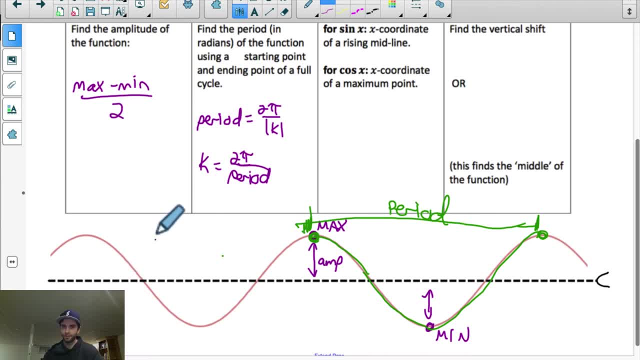 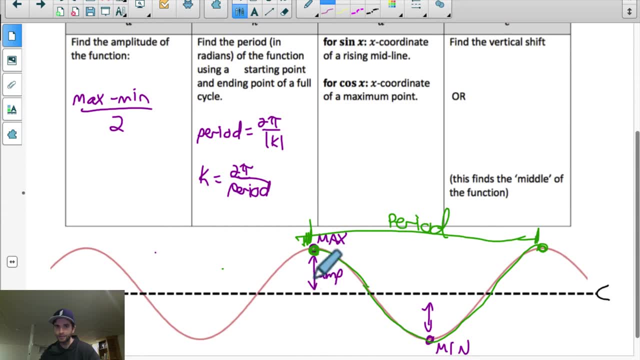 So if we can figure out where the middle is, then we know where the c value is, We know what the c value is. So there are a couple of ways to do this If I want to figure out this c value. well, if I know the max, 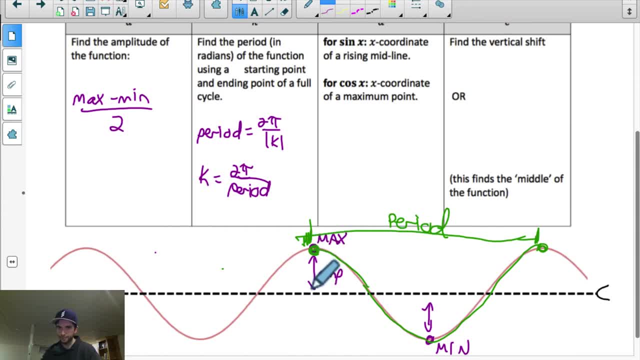 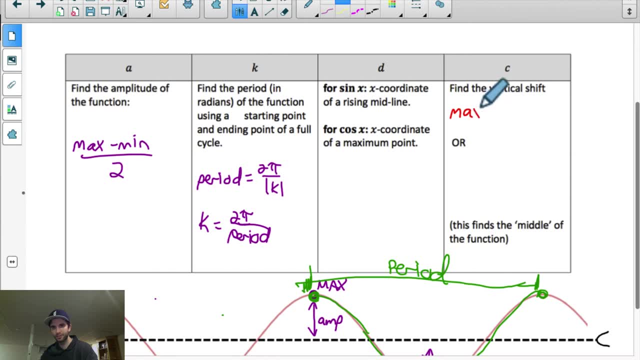 and I know the c value. well, if I have the y value of the max, subtract the amplitude, it tells me the c value. So we can just do max minus amplitude. So I could do max minus the amplitude, Or another way of thinking about it. 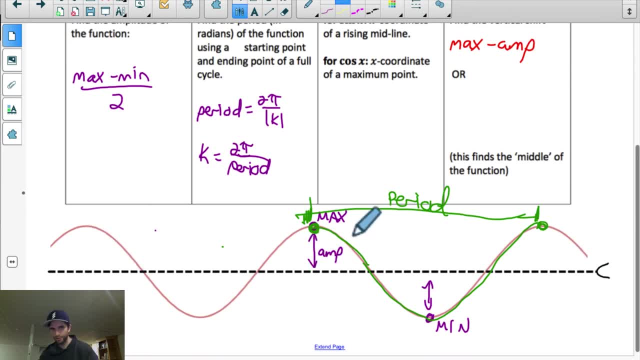 if we want. we know the c value is in the middle of the function, so we just have to find the middle of the max and min. So we need to find the average of the two of them and we can average them just by adding them. 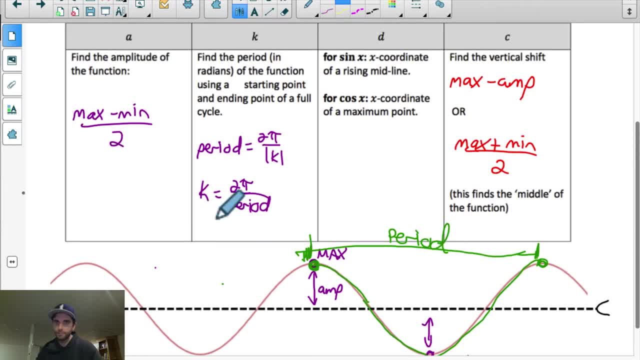 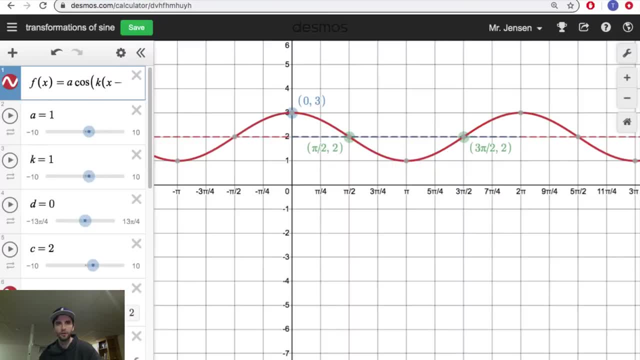 and dividing by 2.. Now let's talk about the most difficult part of this is figuring out the horizontal shift. So let's very carefully look at Desmos first. Okay, so remember the d value is the horizontal shift of the function. 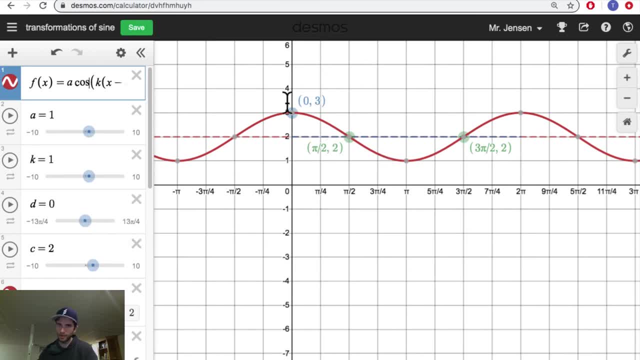 So right now I have a cosine function where the d value is zero. It hasn't been horizontally shifted at all And notice what's on the y axis. On the y axis is a maximum point And if I horizontally shift this function, let's say pi over 2 to the right. 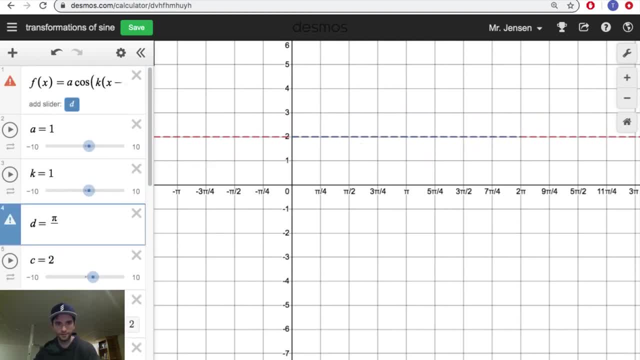 if I move this pi over 2 to the right, make the d value pi over 2, notice where is the maximum point. now It's at an x value of pi over 2.. If I shift this function pi to the right, 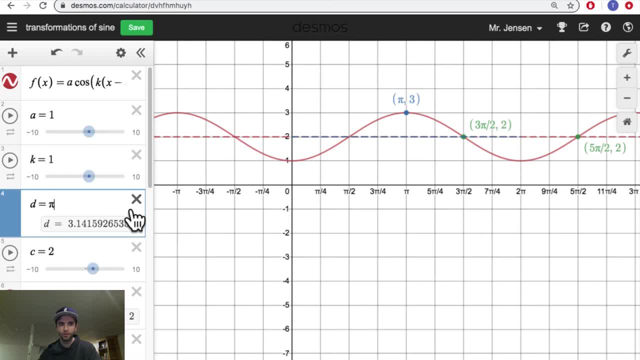 where's the max value now? It's at an x coordinate of pi. So what I want you to notice here is, if we know the x coordinate of a max, we know what horizontal shift has happened. I know there's an infinite number of max points, right? 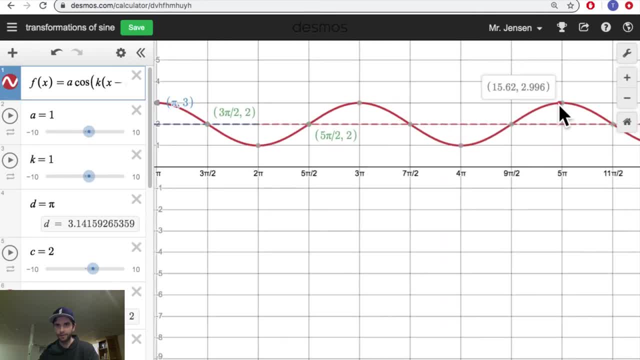 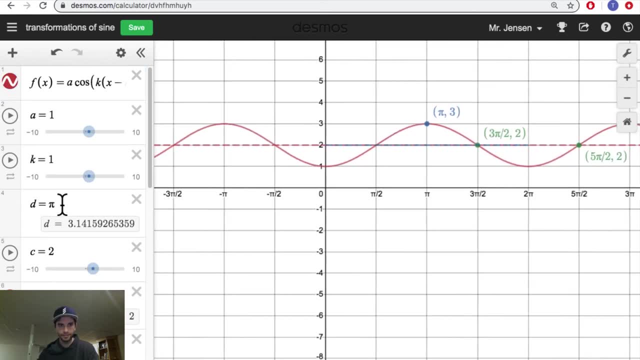 There's a max point there. There's a max point there. I could use the x coordinate of any of those. I could do 5 pi, 3 pi pi. it doesn't matter, right, If I change this to 3 pi. watch what happens to the function. 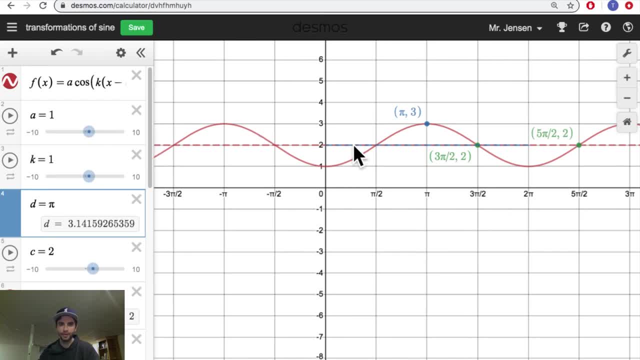 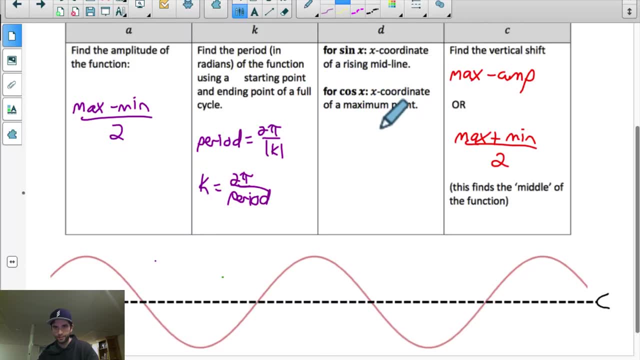 Nothing, It looks exactly the same. It wouldn't matter, As long as we use an x coordinate of a maximum point. then we know the horizontal shift of the cosine function. So that's summarized right here. So if we're trying to write the equation of a cosine function, 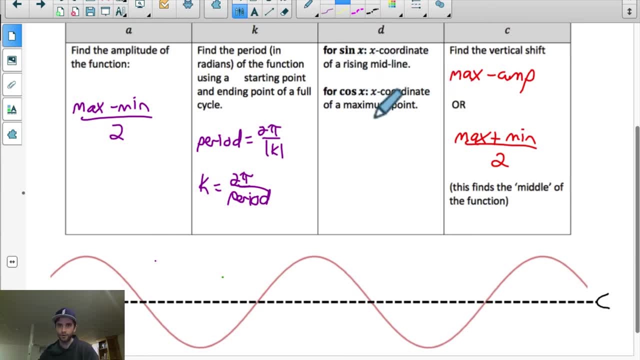 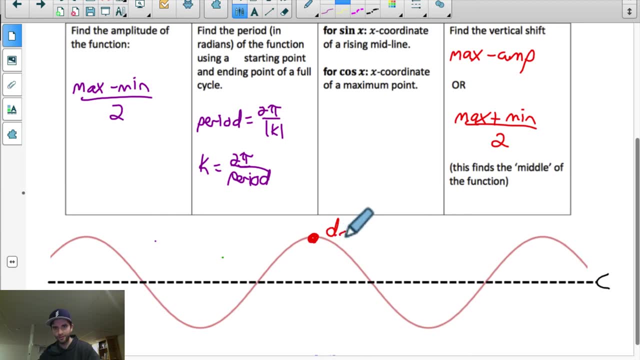 and we want the horizontal shift, the d value. we're just looking at what's the x coordinate of a max point. So we find a max point and we look at what's the x coordinate of that point and that is the d value. 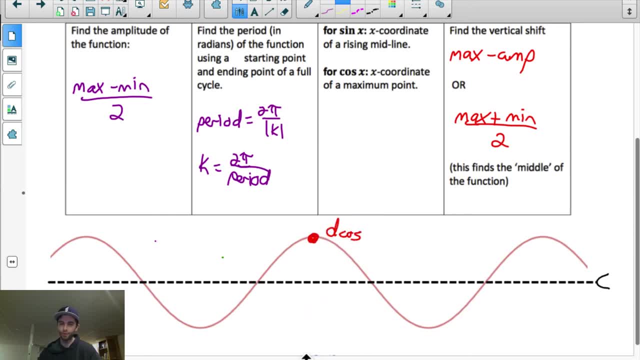 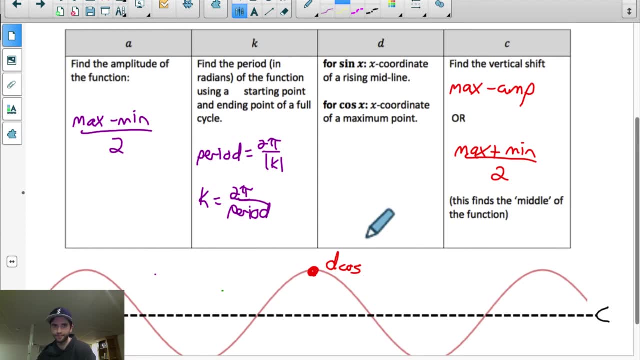 So this would be the x coordinate of this point would be the d value if we were writing a cosine equation. So I'll call that d value for cos. If we were trying to figure out the horizontal shift for a sine function, well, let me change this to a sine function. 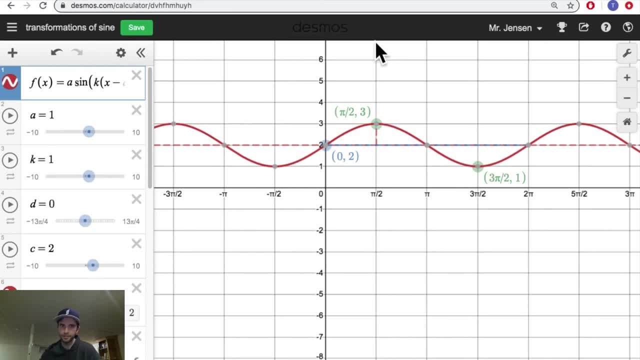 So this sine function hasn't been shifted left or right at all yet. And notice what's on the y axis right now. It's not a max point. It's what we call a right axis. It's what we call a right axis. 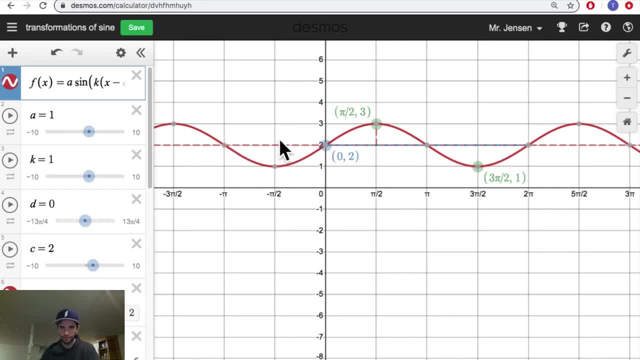 So we're going to call it a right axis. So we're going to call it a right axis, So we're going to call it a rising midline. Here's the midline of the function and here's a rising side of a sine function. 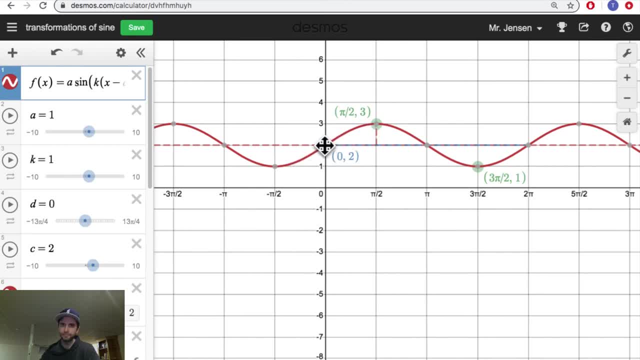 Notice the middle of that rising side, this point right there, so we'll call that the rising midline is on the y axis And as I shift this function left and right, notice that that rising midline is moving. So we have to look for what's the x coordinate of that rising midline. 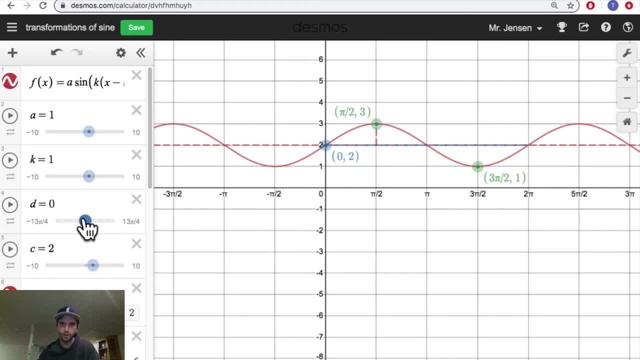 if we want to be able to describe what horizontal shift has happened. If I make this, If I make this, the d value pi over 2, so that shifts it pi over 2 to the right notice. what's the x coordinate of this rising midline? 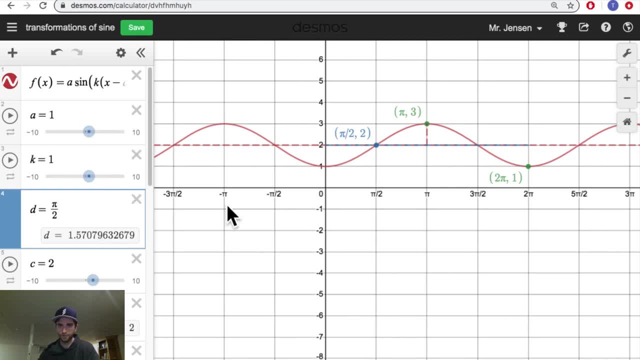 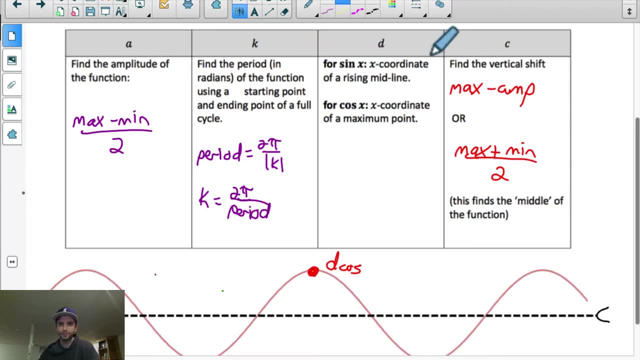 it's pi over 2.. So if we find the x coordinate of a rising midline, we know what horizontal shift has happened to a sine function And that's summarized right here for you. For sine x, if we want the d value. 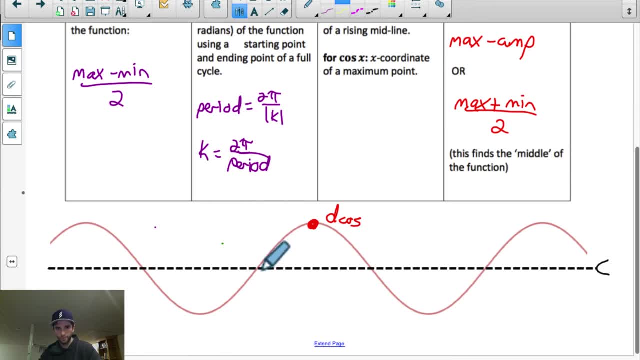 we're looking for. what's the x coordinate of a rising midline. So, reminder, a rising midline is where a midline intersects a rising line, So that would be a point right here. This would be a falling line, right. 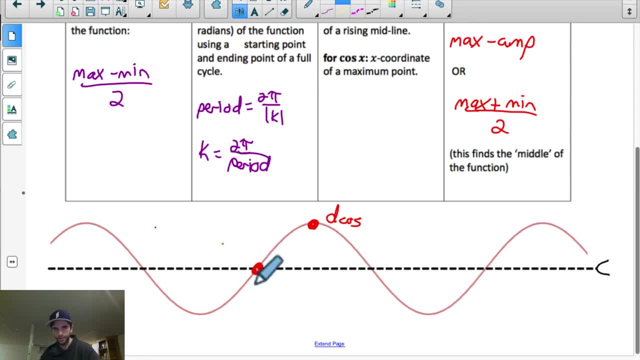 We want a rising midline. So this point right here: If we know the x coordinate of that point, that's the d value for a sine function, That's where the sine function has been shifted And, like I said, we can write. 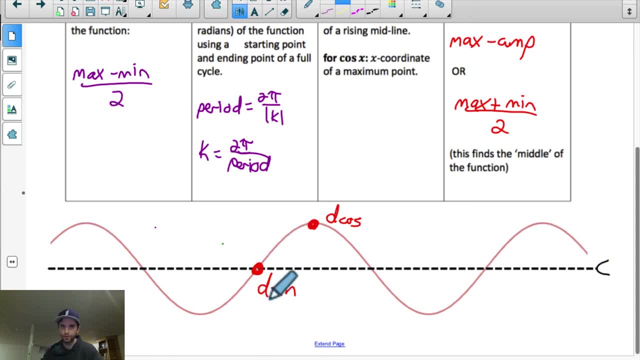 When we have any sinusoidal wave, we could write the equation as a sine or a cosine function just by manipulating the shift that's happened. So we can do that just by looking. If we want to write a sine equation, we just write the x coordinate of one of these points. 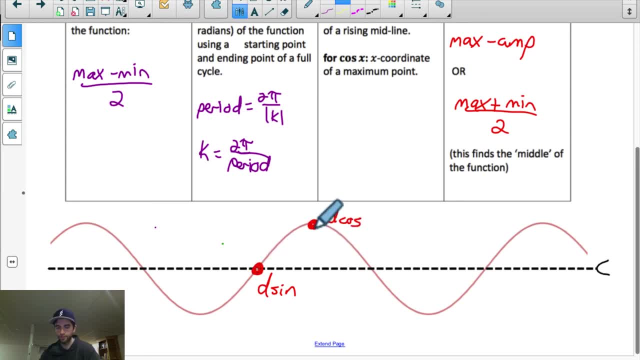 If we want to write a cosine equation, we just write the x coordinate of one of these points, And if I know either of these points, I should be able to come up with the other one by looking at the relationship between these two points. 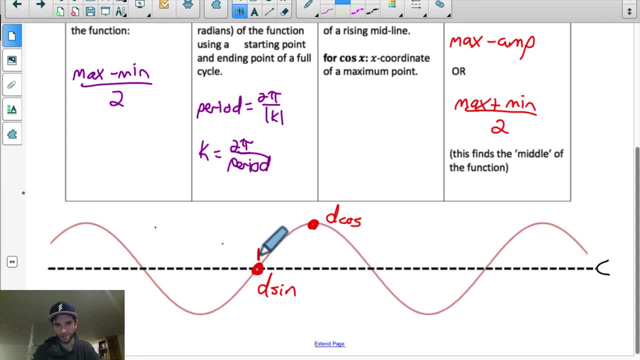 Another important thing I want to talk to you about is the horizontal distance between a rising midline point and a max point. So the horizontal distance between any rising midline and its closest max. they're always going to be pi over 2k apart, right? 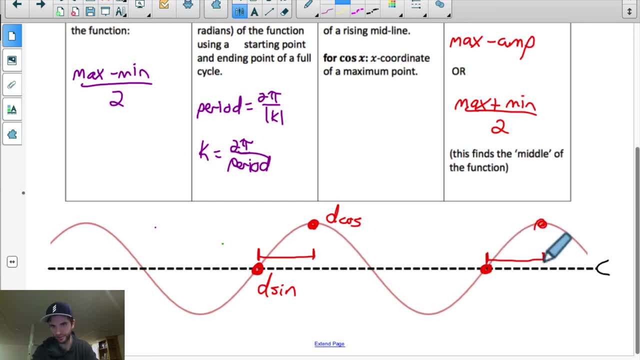 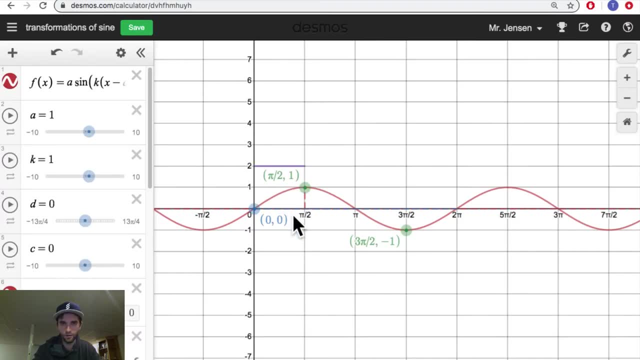 That length of that line. I drew there the horizontal distance between here and here. it's always going to be pi over 2k apart, And let me show you that in Desmos. So notice, here's the sine function. If we look, notice the scales going up by pi over 2s. 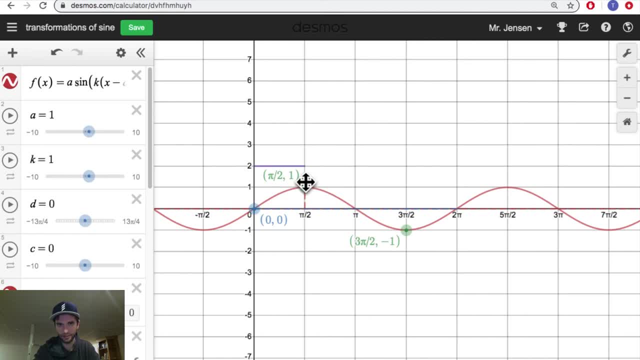 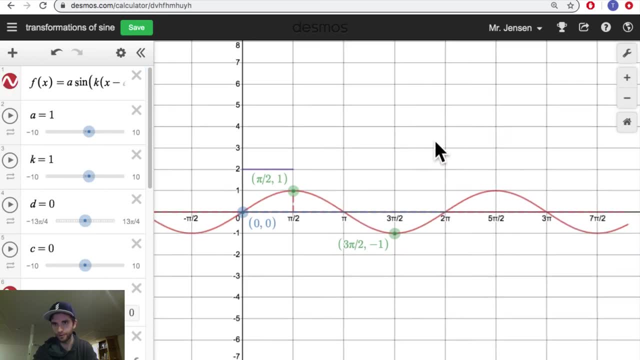 Well, what's the distance between any rising midline here and its closest max? One unit pi over 2.. How about between this rising midline and this max? One unit, so another pi over 2.. And that's true between any rising midline and its closest max. 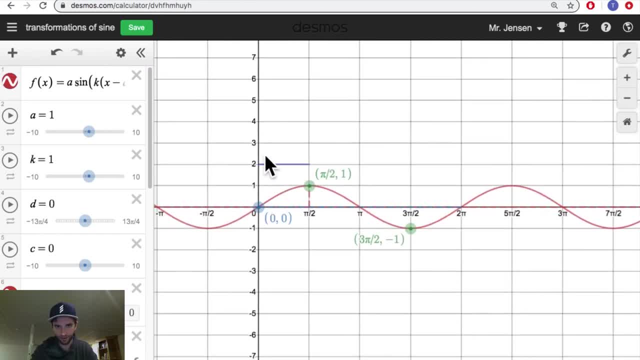 they're always pi over 2 apart, And I have that distance represented with this purple line up here. So the distance between the two points is always pi over 2, unless there's been a horizontal stretch or compression, And the horizontal stretch or compression is always done by a factor of 1 over k. 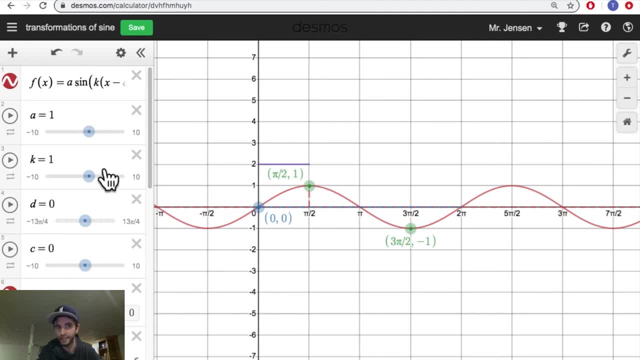 So we have to figure out the distance by doing pi over 2 over k, which could be summarized by pi over 2k. Notice, as I manipulate k, the horizontal distance between the rising midline and the max is changing, So this summarizes the distance between the two. 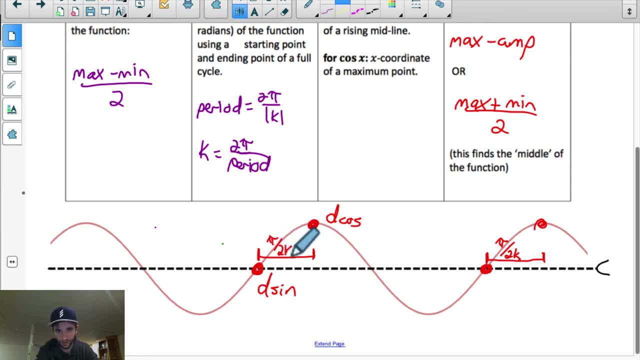 The distance between the two is always pi over 2k. So let's say I knew the x-coordinate of this point and I wanted the x-coordinate of this point. So if I wanted the d-value for cosine, I could calculate it by doing the x-coordinate of this point. 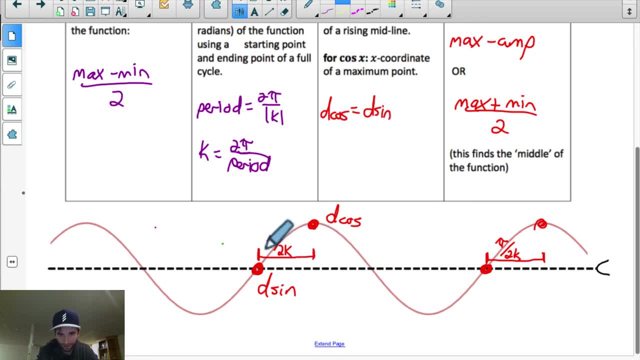 which we've summarized as the d-value for sine, and then adding this horizontal length, So adding pi over 2k. So this is going to be an important formula. And what if I wanted to calculate the d-value of sine and I knew the d-value of cos right? 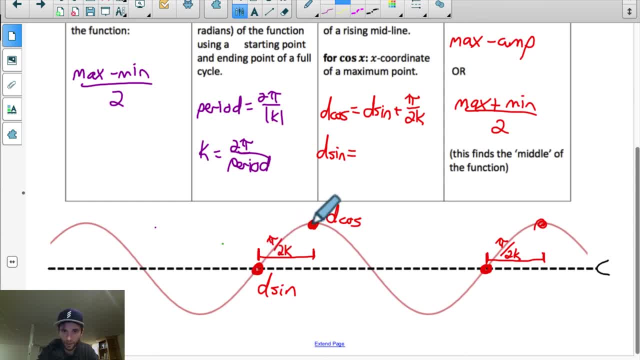 What if I knew this, this x-coordinate, but didn't know this x-coordinate? Well, I know the distance between the two is pi over 2k. So I take this x-coordinate, subtract pi over 2k, it brings me to this x-coordinate. 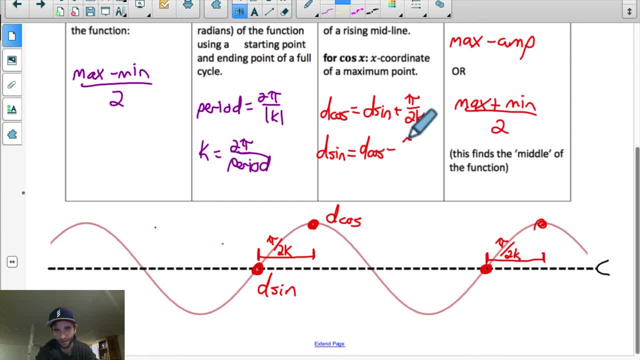 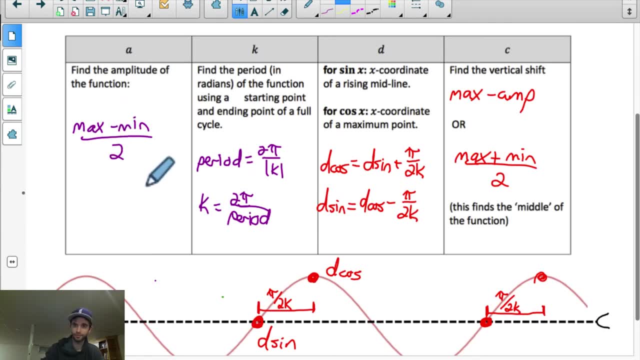 So I would do d cos minus pi over 2k. So I think that's all of the properties we need to be able to generate the equation from a graph. Let's give it a shot. So, this graph, we're going to write a sine and a cosine equation that describes this function. 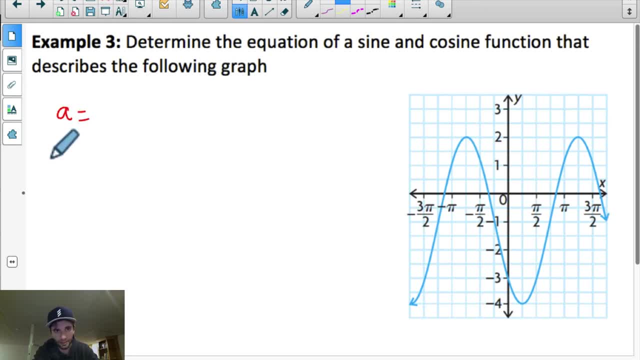 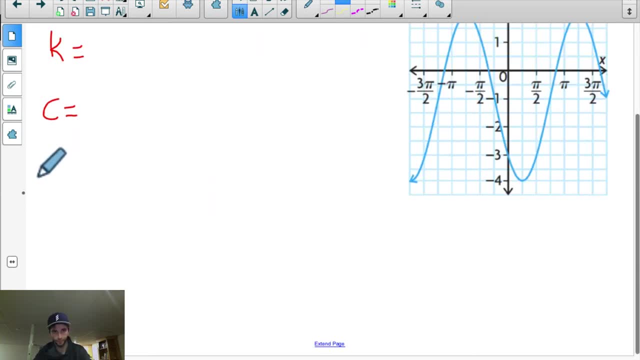 So we're going to need to find all four parameters- a, k, c- and then, since we're writing both a sine and a cosine function for this graph, we're going to need two different d-values. right, The d-value is the only one that's different, depending on whether we're doing a cosine. 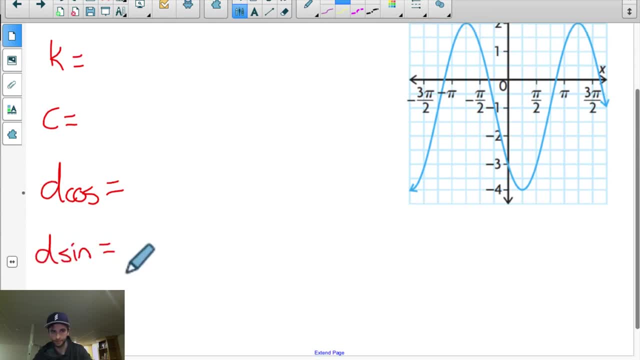 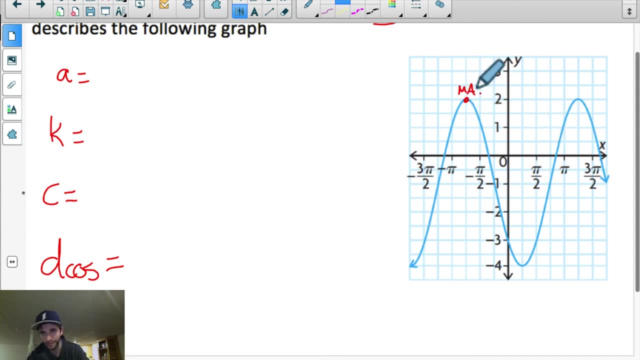 or a sine function. So let's start with a. a is amplitude And we can calculate the amplitude by doing the max minus the min over 2, right, Amplitude is half the distance between between max and min. So we just do max minus min over 2.. 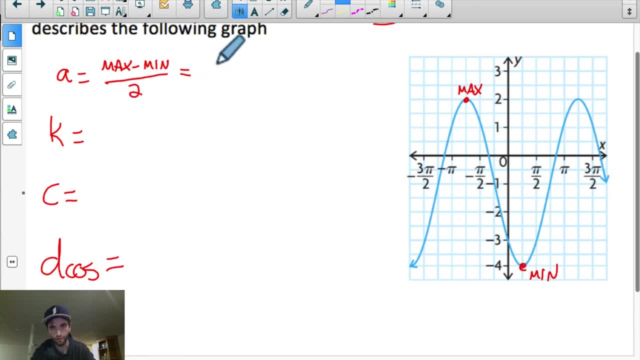 And that will tell us half the distance between the max and the min. So the max y value is 2 minus the min y value is negative 4.. Cut that in half, 6 over 2 is 3.. So our amplitude is 3.. 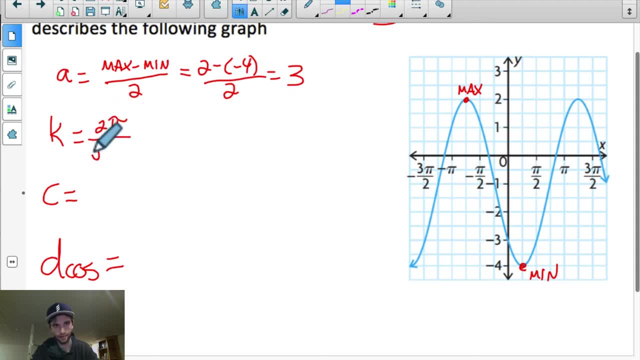 k. we calculate by doing 2 pi divided by whatever the period of the function is. So we need to map off one cycle of this function and figure out the horizontal length of that cycle, And then that's the period of it. So here's one cycle. 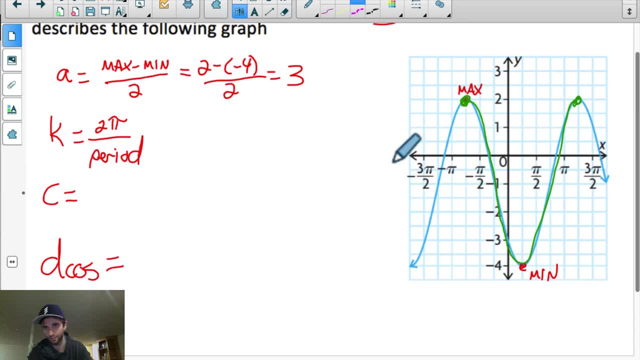 I'll map it off in green. So between max points is one cycle. Now I need to figure out what is the horizontal length of that cycle. What horizontal distance have I covered between those maximum points? So it'll be useful to figure out what is the scale going up by. 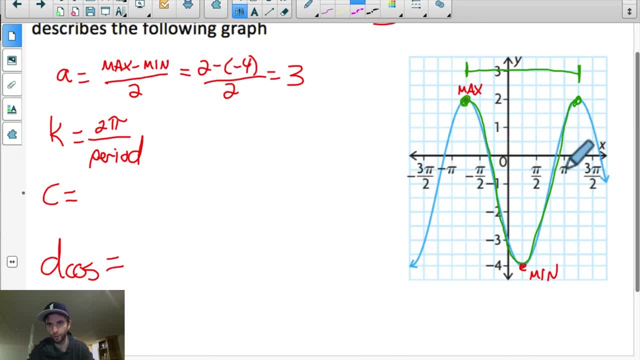 Well, where's pi? Pi is right here? It's at the 1,, 2,, 3, 4th spot. That must mean I'm going up by pi over 4.. 1 pi over 4, 2 pi over 4,, 3 pi over 4,, 4 pi over 4.. 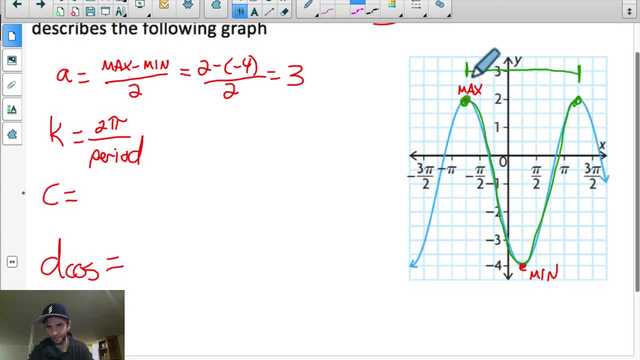 So each unit is pi over 4.. So let me do that. Let me count the length of this cycle: 1 pi over 4,, 2 pi over 4,, 3 pi over 4,, 4,, 5,, 6,, 7,, 8.. 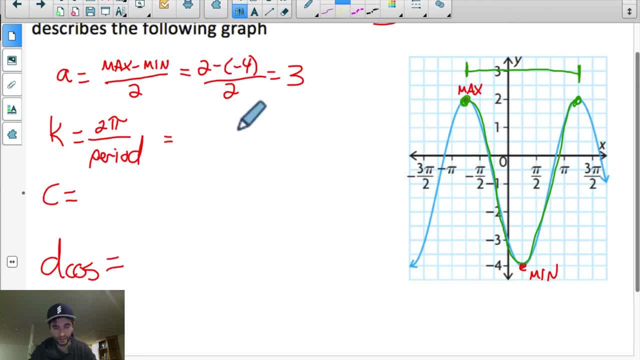 It's 8 pi over 4, which is 2 pi. So the period is 2 pi. So 2 pi divided by 2 pi is 1.. There's been no horizontal stretch or compression. that's happened. That's why the k value is 1.. 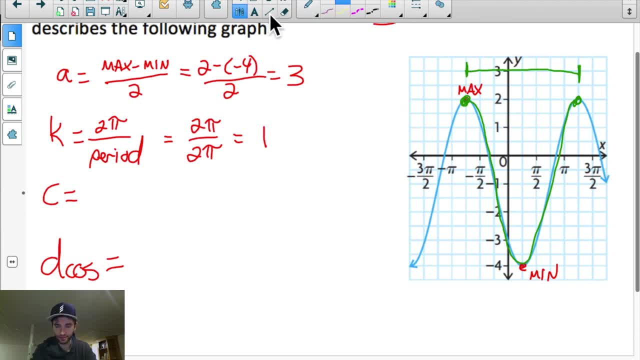 C I'm looking for where is the midline of this function? And remember, the midline is halfway between the max and the min, So I just have to average them. I just have to do max plus min over 2.. Max is at 2.. 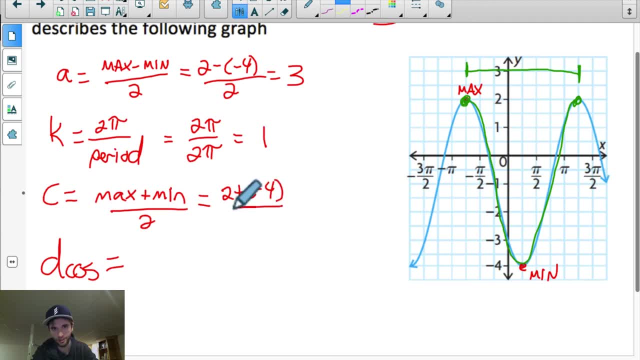 Min is at negative 4.. 2 plus negative 4 over 2.. So the middle of those two points will give me negative 1.. And if I were to draw a midline of this function, it would be at negative 1, at a y value of negative 1.. 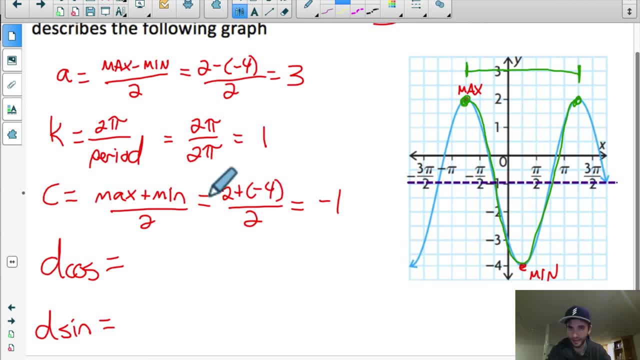 So my c value is negative 1. Notice how that splits the function in half. It splits the function in half horizontally. Now, if I want the d value for cosine, I'd be looking at what's the x coordinate of a maximum point. 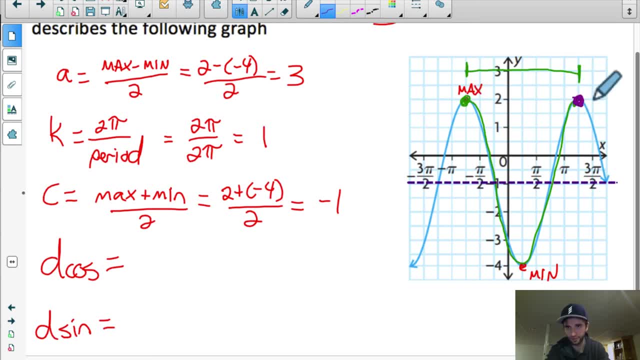 So I could use any maximum point. I could use this one, I could use this one. It doesn't matter, So I'll choose this one this time. So what's the x coordinate of this point? It's at the fifth tick mark. 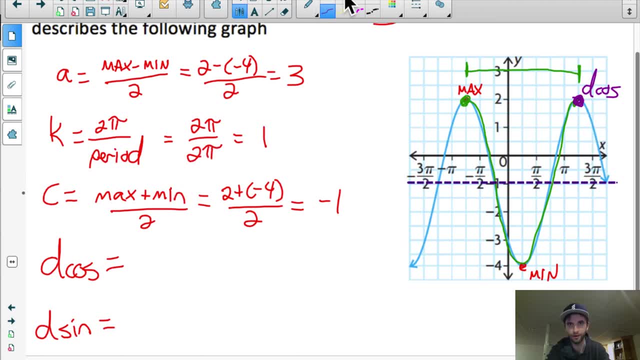 So fifth unit, each unit is pi over 4.. So it's at 5 pi over 4.. So d cos 5 pi over 4.. The cosine function has been shifted 5 pi over 4 to the right The d value for sine. 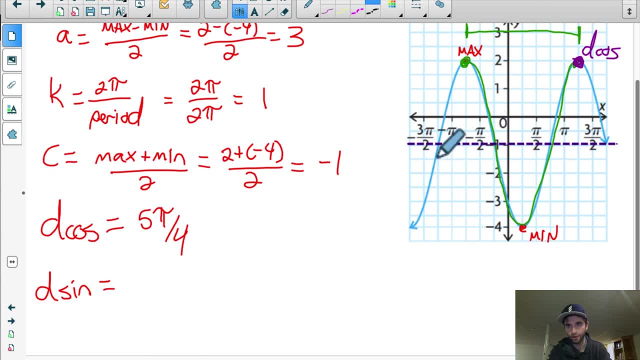 I'm looking for. what's the x coordinate of a rising midline? So here's the midline, Here's a rising line. Therefore, here's a rising midline, The x coordinate of that is the d value for sine And the x coordinate of this point. it's at the third unit: 1,, 2,, 3.. 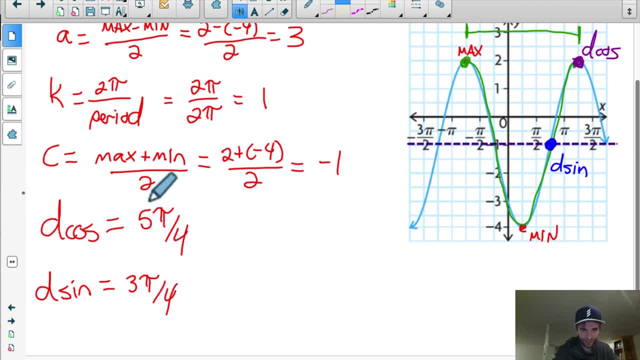 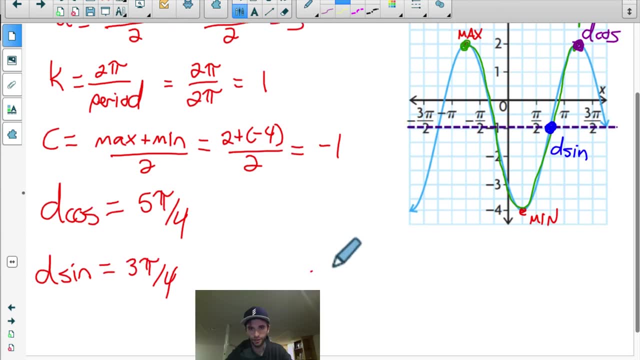 So that's 3 pi over 4.. And notice what's the difference between those two values. The difference is 2 pi over 4, pi over 2, right, They're pi over 2 apart. So now I can write my equations just by plugging. 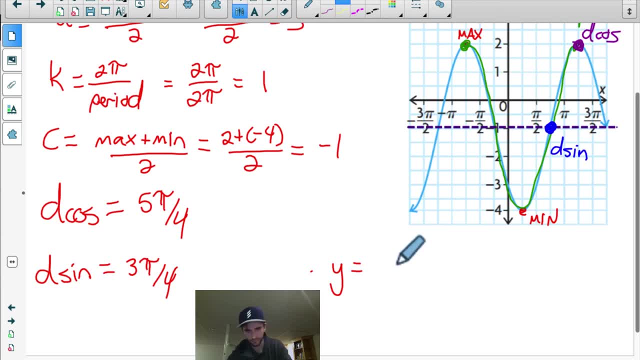 in my a, k, d and c parameters. So y equals 3.. I'll do the cosine function first: x minus 5, pi over 4 plus the c value of negative 1. And my sine function is going to look exactly the same. 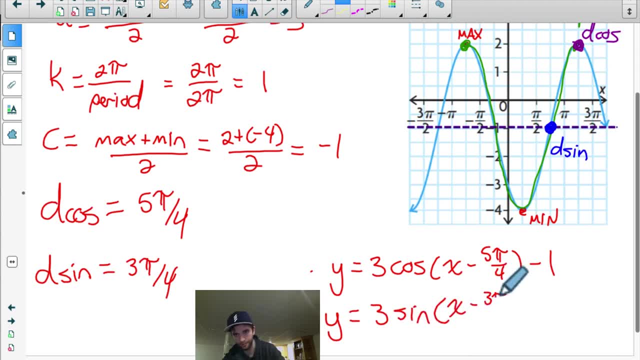 except for the d value is different. It's x minus 3 pi over 4 minus 1.. This function and this function are equivalent to each other. They both would give me this graph right here. Let's try one more: Determine the equation of a sine and cosine function that describes this graph. 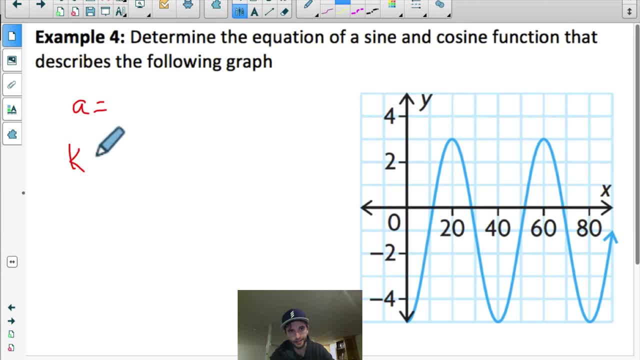 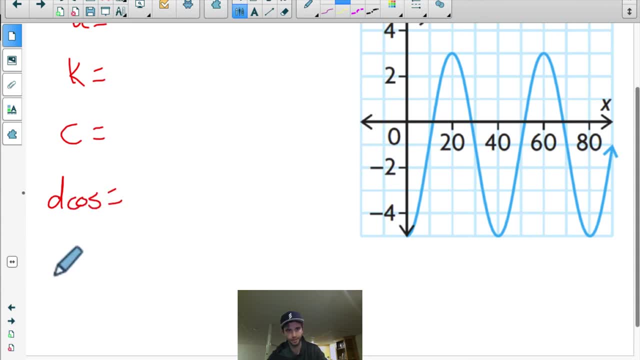 So let's find a k, c, And then we're doing a sine and a cosine function again. So I'll need the d value for cosine And I'll also need the d value for sine. So let's start with a amplitude. 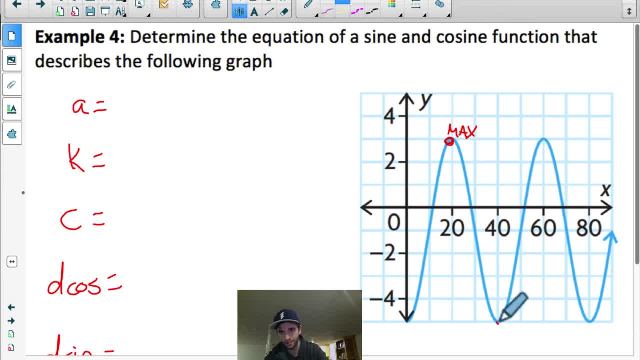 Amplitude's half the distance between max and min. So I need half the distance between 3 and negative 5.. So I'll find the distance between 3 and negative 5 by subtracting them And then cut it in half. So 3 minus negative 5 is 8, divided by 2 is 4.. 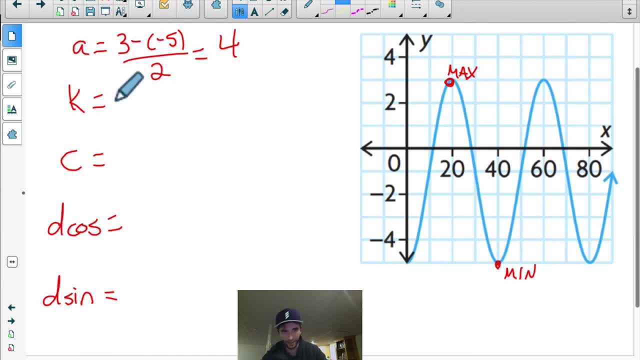 So the amplitude is 4.. The k value: I can calculate that by doing 2 pi divided by whatever the period of this function is. So let's map off one cycle. I'll do it between maximum points. It doesn't have to be between maximum points. 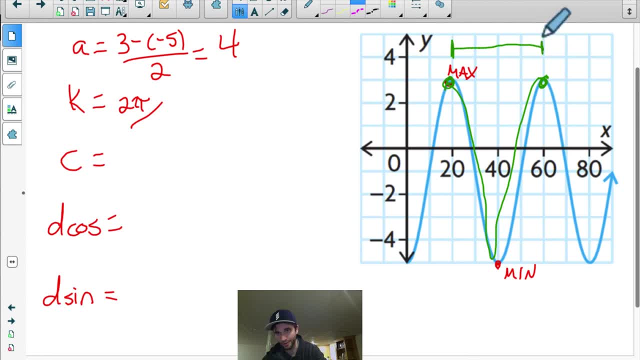 I just find that easiest. So what's the horizontal length of this? So our scale is going up by 10.. 10, 20,, 30,, 40. The horizontal length of this cycle is 40. So my k value, if I reduce this, is pi over 20.. 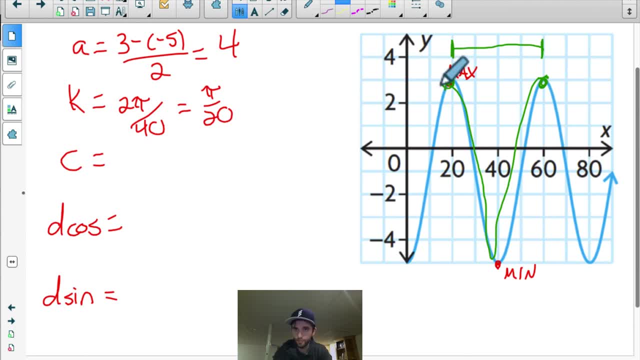 The c value is going to be where's the midline of this function? And I can figure that out by knowing it's going to be halfway between max and min. So it's the average of the max and the min, So 3 plus negative 5 over 2.. 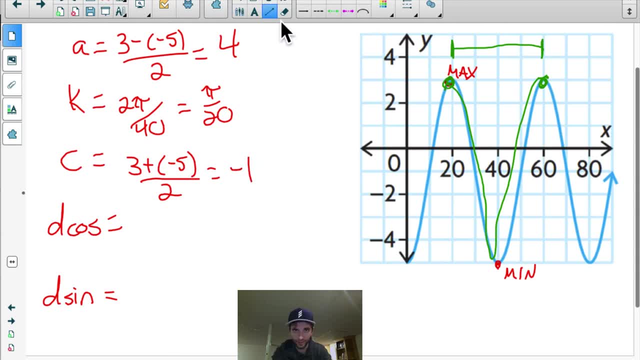 That's negative 2 over 2, which is negative 1.. So the midline is at negative 1 again. Let me just draw that quickly. And the d value for cosine is going to be the x coordinate of a maximum point. 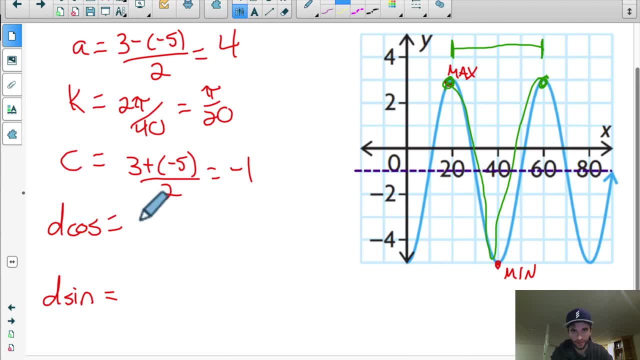 So here's a maximum point. Its x coordinate is 20.. So the d value for cosine is 20.. The cosine function has been shifted 20 to the right, because the max used to be on the y-axis, Now it's over here. 20 to the right. 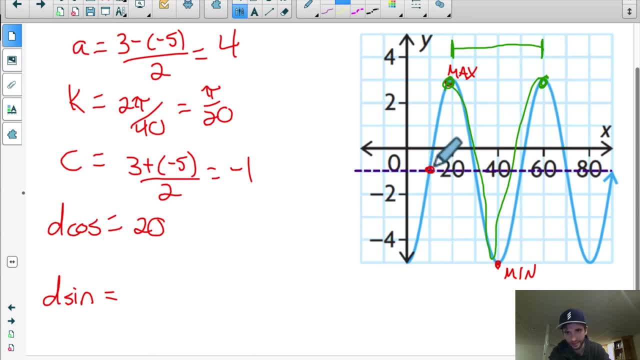 d value for sine. I'm looking for the x coordinate of a rising midline. So I'm looking for the x coordinate of where a rising line intersects a midline. So either that one or that one, Or there's an infinite. There's a number of them. 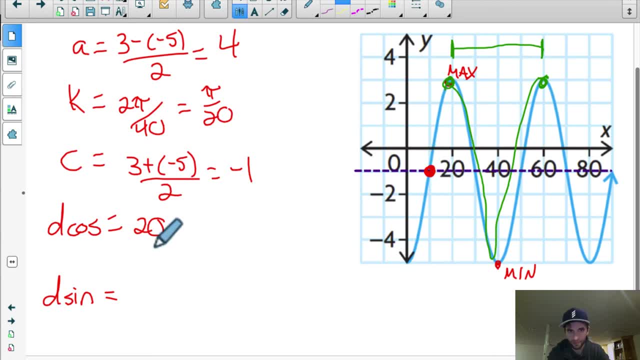 I'll just choose the one closest to the y-axis, This one right here. the x coordinate of that point is 10.. Notice the difference between these two points. is pi over 2k. Let me demonstrate that to you. What is pi over 2k? 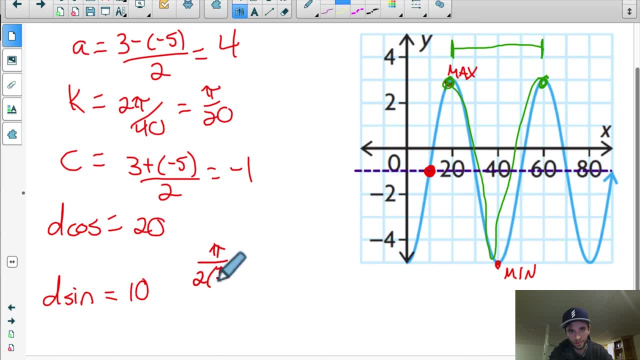 What's pi over 2 times pi over 20?? So that would be pi over 10.. Flip and multiply, That's 10.. The distance between an x value of a max and an x value of a rising midline is always pi over 2k apart. 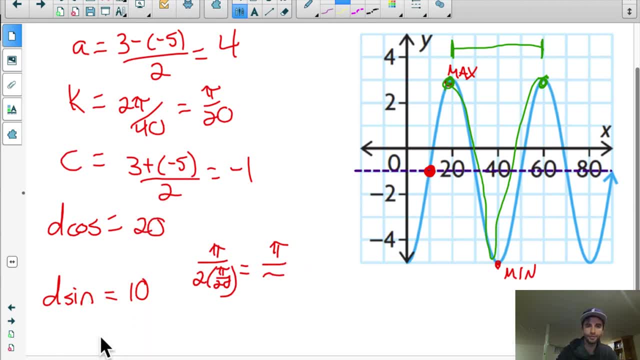 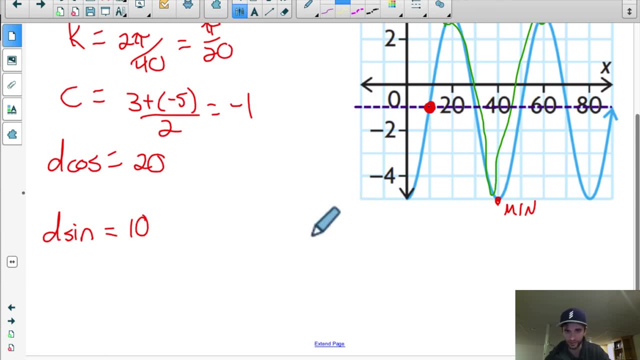 So they're 10 apart. So let's write the equations now for this function And we can write a sine and a cosine function that are both equivalent to each other. So I'll start by doing the cosine function. So y equals 4 cos and I have a k value this time. 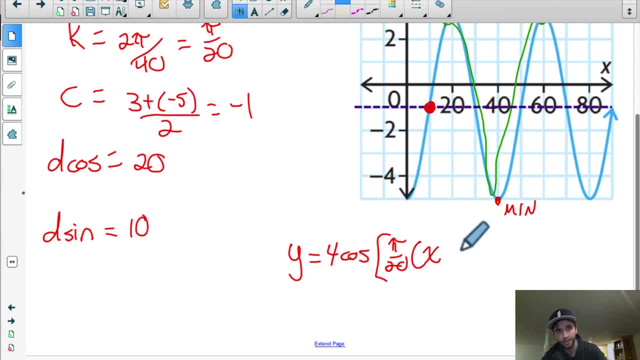 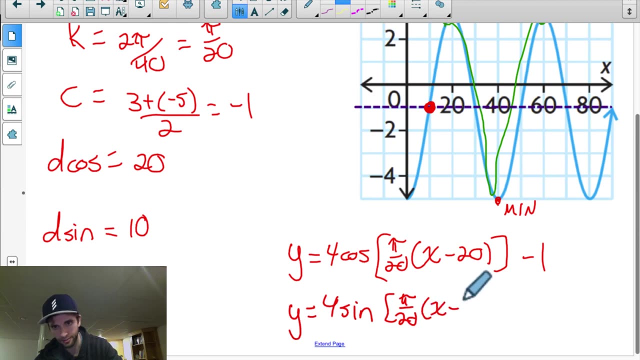 so pi over 20,, x minus 20,, plus the c value, which is negative 1.. And now I'll do the sine function as well, where everything is exactly the same except for the d value. So same k value, but now it's x minus 10, minus 1.. 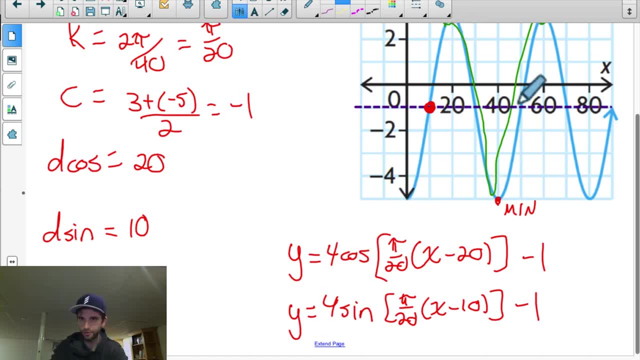 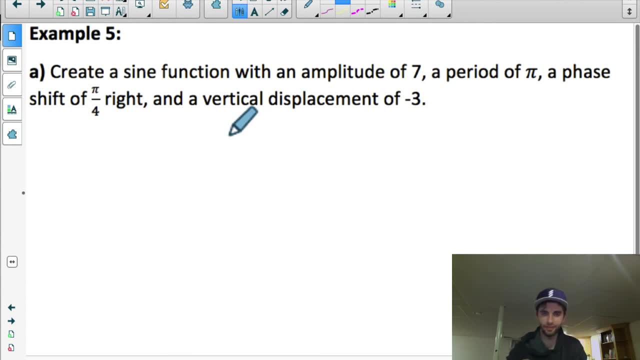 So those two equations are equivalent. They both match up with that function right there. How would, if we didn't have the graph? We only had information in words? This is where we're going to have to use the relationship between the d value for cos and sine. 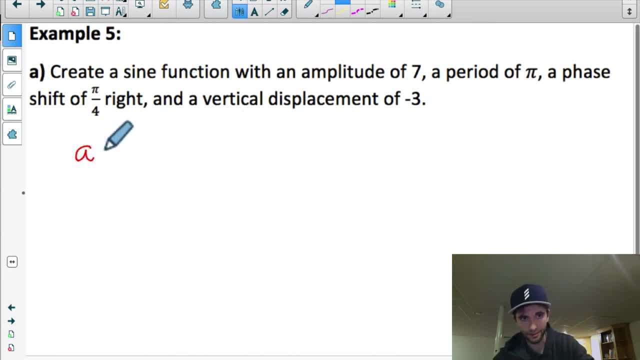 So create a sine function with an amplitude of 7.. Okay, well, that tells me. the a value is 7, a period of pi. so i can calculate the k value by doing 2 pi divided by the period, i get k is 2.. a phase shift of pi over 4, right, okay, well, it tells me. 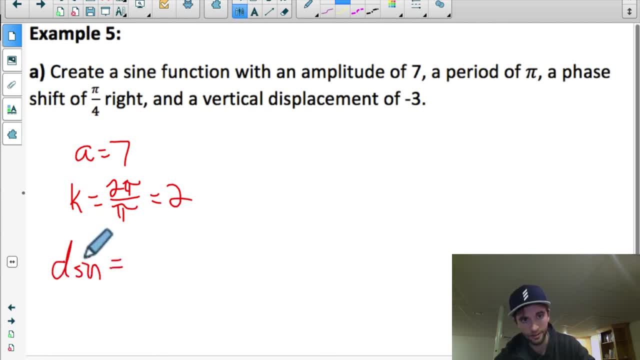 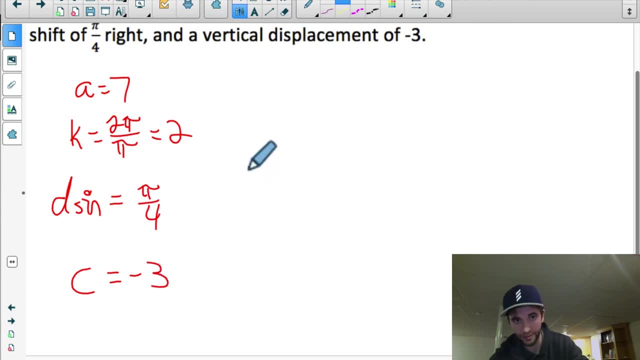 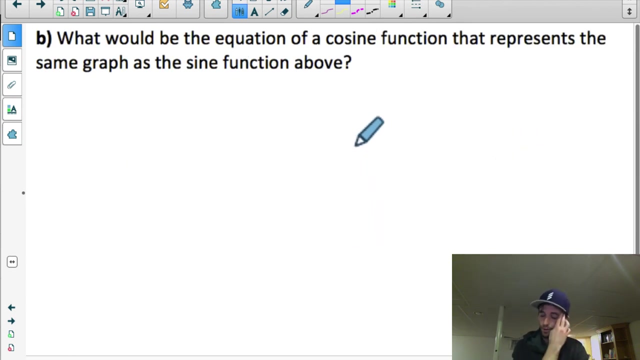 it's a sine function. so the d value for sine is pi over 4 and a vertical displacement of negative 3. that just means down 3, so my c value is negative 3.. so it's easy to write my sine function: it's just 7 sine 2 x minus pi over 4 minus 3.. part b of this question is the more difficult part. 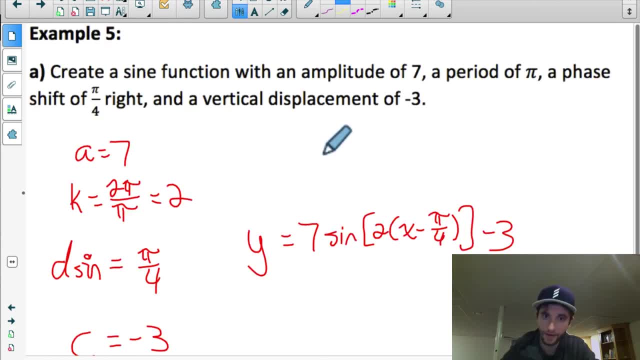 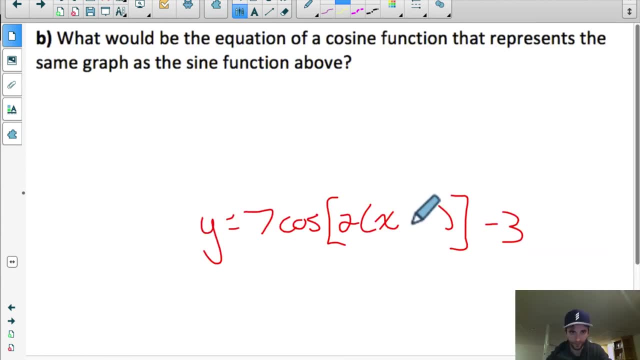 what would be the equation of a cosine function that represents the same graph? well, i know the a, k and c values are going to be exactly the same. so how do i figure out the d value of the cosine function? well, i have to know where is a maximum point, right? the 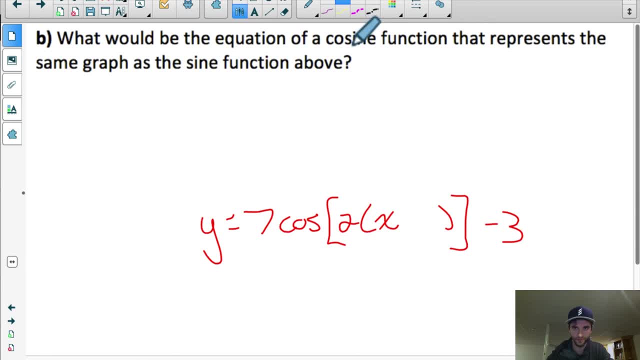 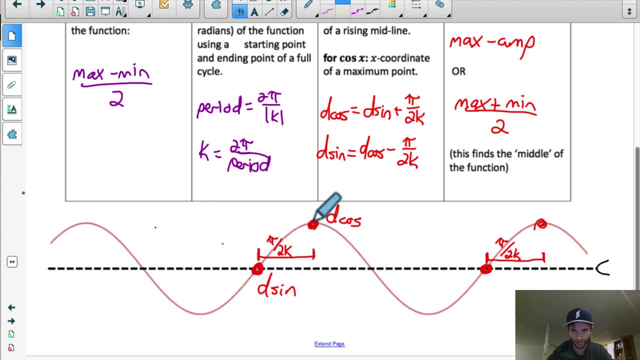 x coordinate of a max is going to tell me the horizontal shift of a cosine function. and let's say, think back to this graph i showed you earlier. well, if we know the x coordinate of this, we could figure out the x coordinate of this just by adding pi over 2k. that's what it tells me. 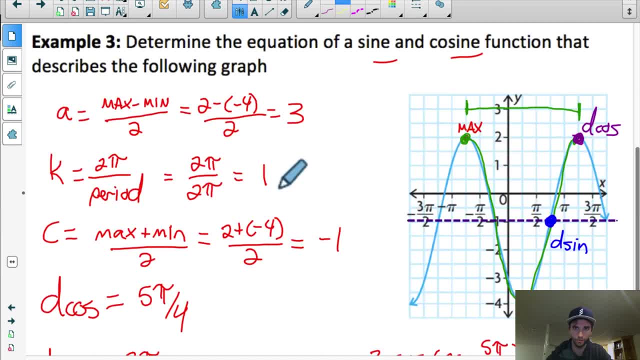 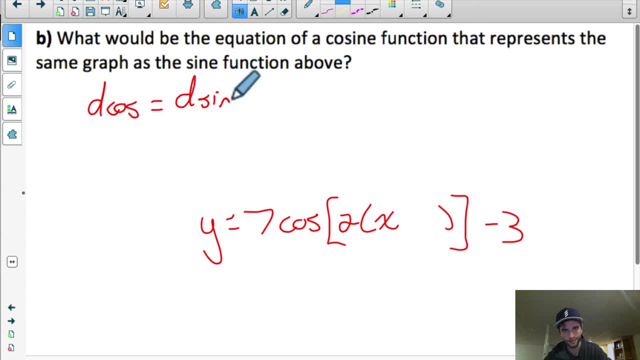 right here. if i want the d value for cos, take the d value for sine, add pi over 2k. so let's do that here. if i want the d value for cos, we take the d value for sine and we add pi over 2k. so in this case the d value for sine was pi over 4. 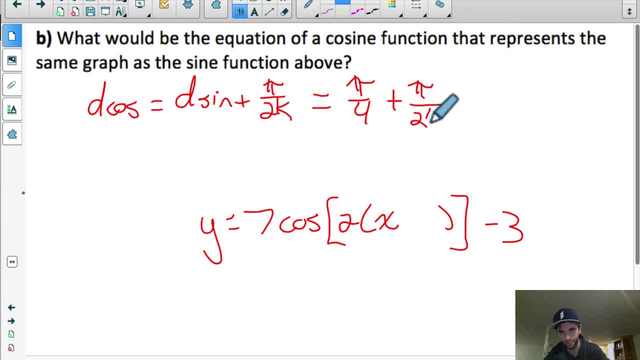 and we add pi over 2 and the k value was 2, so we add pi over 4. so pi over 4 plus pi over 4 is 2, pi over 4, which is pi over 2.. so the d value for the cosine function is pi over 2.. so there's an equivalent. 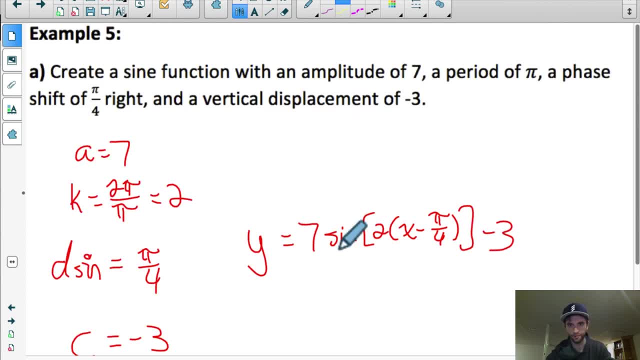 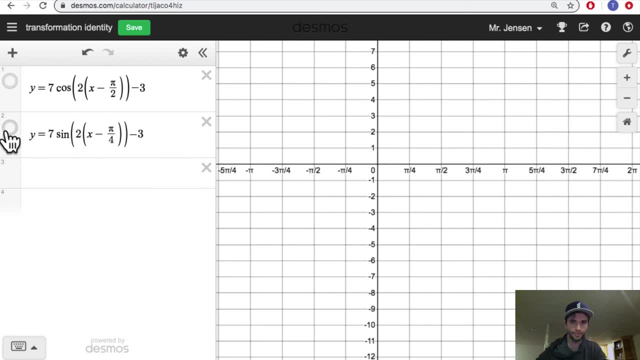 cosine function. so this function and this function are equivalent to each other. they give you the exact same graph. let me just finish off by showing you that in desmos- okay, i have the two equations written here. if i reveal the cosine equation, the functions right there. if i reveal the sine equation, 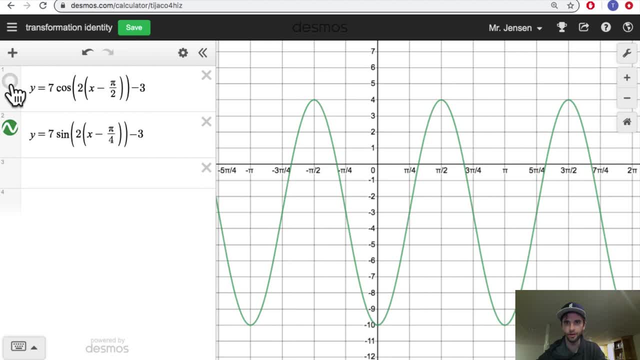 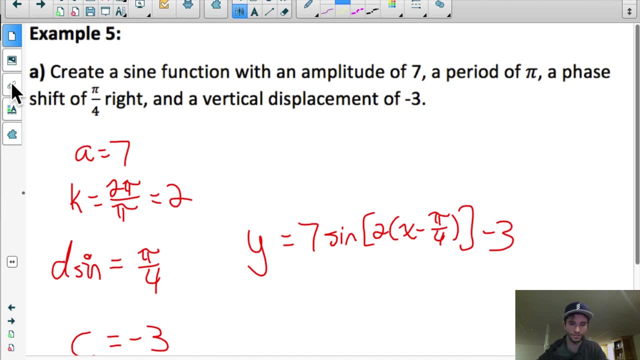 in the exact same spot. notice: they overlap exactly with each other, so they're equivalent equations. uh, two ways of describing the exact same sinusoidal function. okay, so that's it for this lesson. make sure you try the practice questions that go along with it, and that's it.